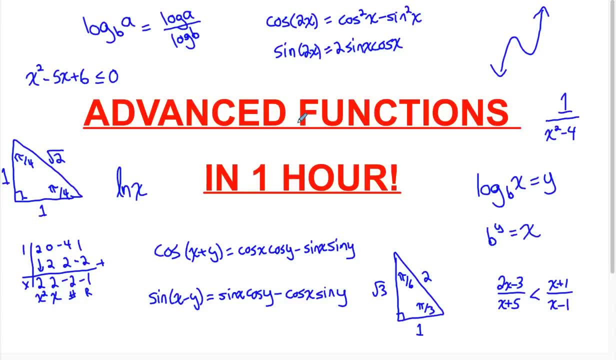 So here's a quick one-hour video that's going to review everything you would have learned in the grade 12 advanced functions math course. So this video is just meant to be a quick refresher for you, heading into your exam, about all of the main concepts you would have learned. This video is going to be divided into three parts: The first part about polynomial functions, the second part about trigonometry and the third part about logarithmic functions and also about rational functions, So polynomial functions. The first thing you would have learned to do is be able to. 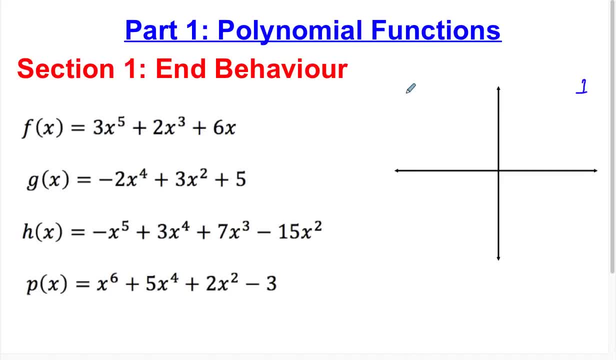 determine the end behavior of a function based on what quadrant number it starts in and finishes in. So you have to remember that the quadrants are numbered 1, 2,, 3,, 4, just like that. And we'll determine the end behavior based on the degree of the polynomial and also based on the sign of. 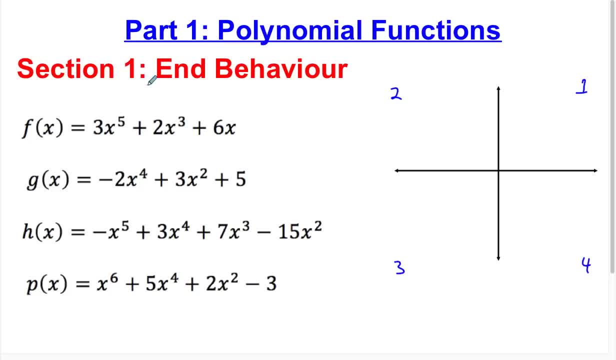 its leading coefficient. So let's start by looking at our even degree polynomials. So the highest degree term is an even degree term. So, for example, degree 4 and degree 6 polynomials, Our even degree polynomials. So let's first look at this one down here: p at x, So it's an even. 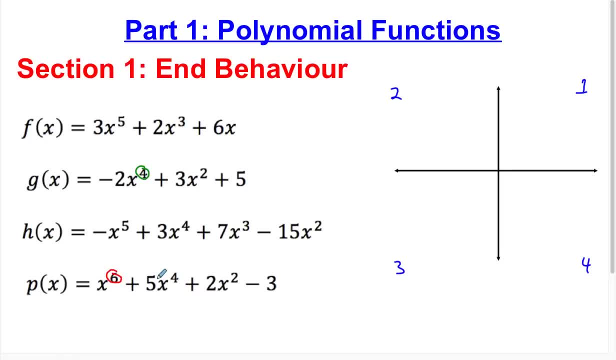 degree polynomial, which tells us it's going to have the same end behavior. So as we go to the right and left, it's going to be going off in the same direction. So how do we know if it's going from 2 to 1 or from 3 to 4?? Well, it depends on the sign of the leading coefficient. This leading 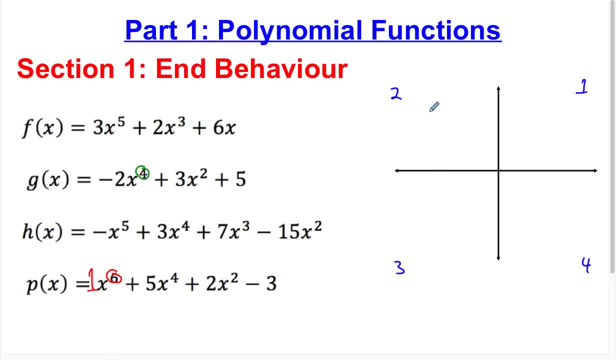 coefficient is positive, It's a positive 1.. So that means our end behavior is going to be going from 2 to 1.. So this is where it's going to start, This is where it's going to finish. It's going to do some. 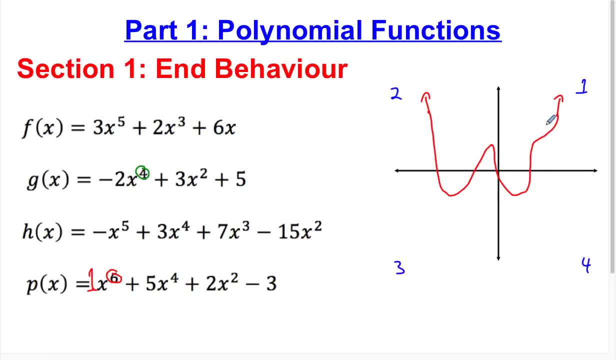 funny stuff in between. We don't know for sure when it's in standard form, but we know for sure it's going to start from 2 and finish in 1.. How about if we have once again an even degree polynomial? So highest degree term is degree 4, but we have a negative leading coefficient. So 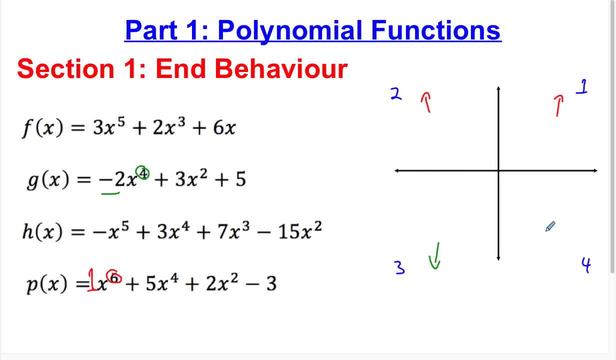 it's once again going to have the same end behavior, but this time it's going to be flipped vertically and it's going to be going from quadrant 3 to 4.. And once again, since it's in standard form, it's going to be in between its end behaviors, But I know for sure it's going to start in 3. 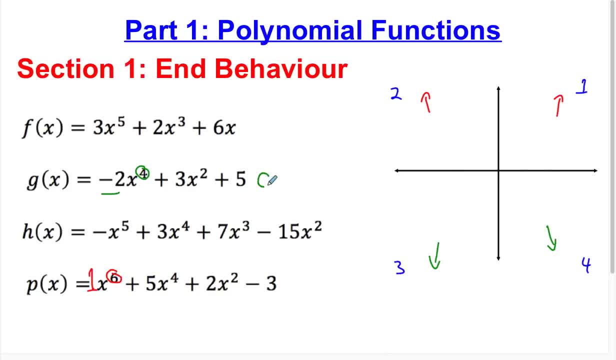 and it's going to end in 4.. So let me just jot down these two end behaviors. So this one is q3 to q4. And this one, the other, even degree polynomial goes from q2 to q1.. So if we have even degree, 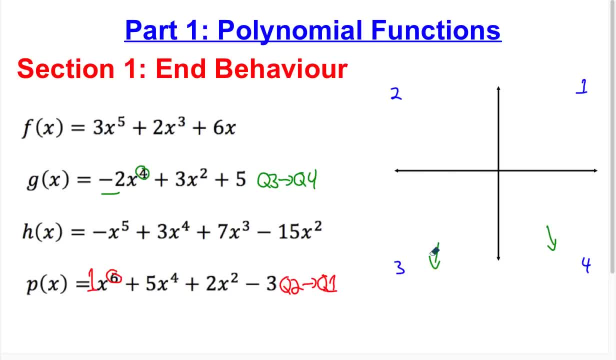 polynomial. it has the same end behavior: Positive leading coefficient from 2 to 1,. negative leading coefficient from 3 to 4.. What if we have an odd degree polynomial? Let's look at these two polynomials, So f of x- odd degree positive leading coefficient- and h of x. 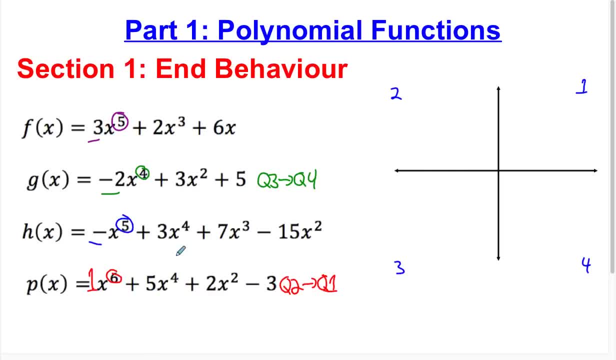 odd degree negative leading coefficient. So odd degree polynomials are going to have opposite end behaviors. So let's look at the one with the positive leading coefficient first: f of x. So it's going to go from quadrant 3 to quadrant 1.. As we go to the left it's going down to negative. 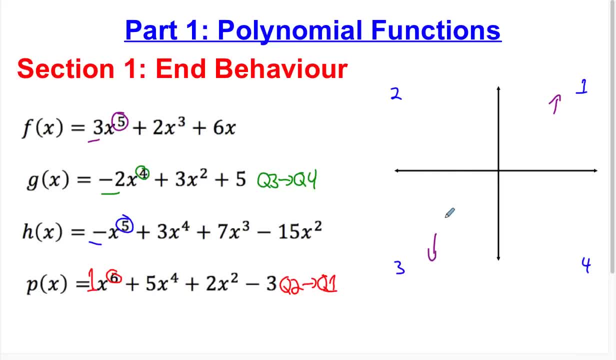 infinity. As we go to the right it's going off to positive infinity. So that's what we call opposite end behaviors, And all odd degree polynomials have this Once again. it's going to do some stuff in between, but we know it's going to start in quadrant 3, finish in quadrant 1.. 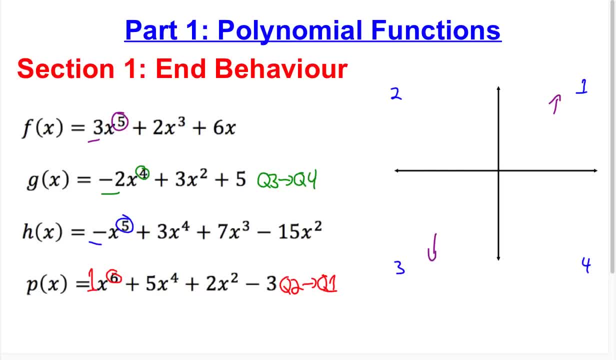 If we have an odd degree polynomial but a negative leading coefficient, it once again has opposite end behaviors: infinity in one direction, negative infinity in the other direction, And it's going to do some stuff in between. We know for sure it's going to go from 2 to 4.. So this one was from 2 to 4.. 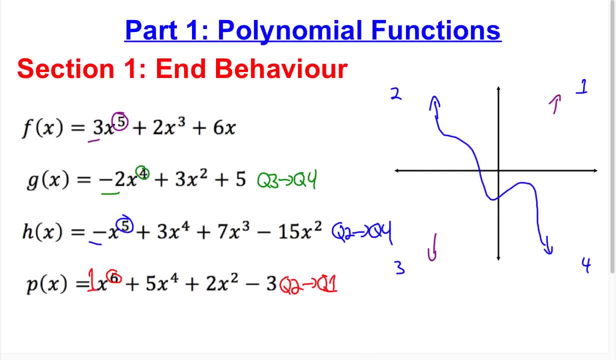 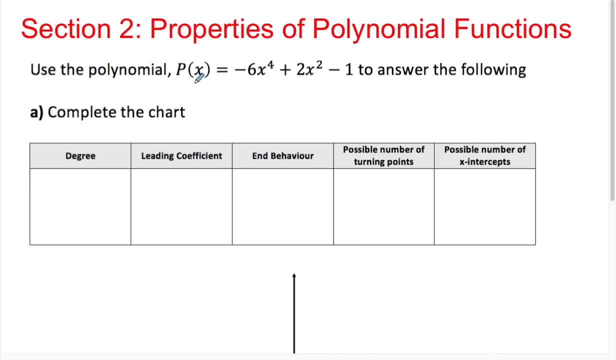 And this one was from 1 to 3.. So we can state the end behavior based on whether it's even or odd degree and whether the leading coefficient is positive or negative. Let's look at this specific polynomial function here. So this polynomial function, 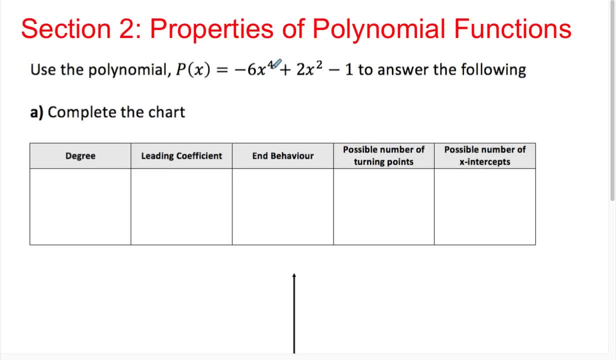 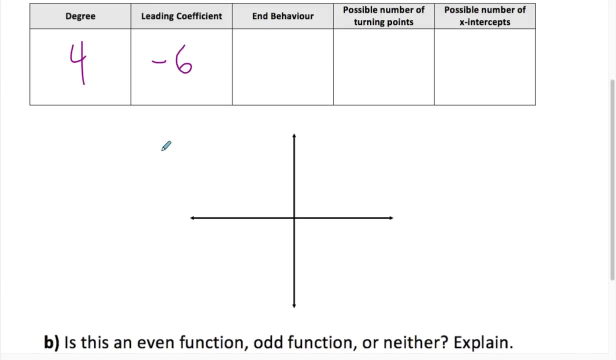 is an even degree polynomial, because the highest degree term is an even degree term, It's degree 4, degree 4 polynomial: The leading coefficient of that specific term is negative 6. So we have even degree, which means it's going to have the same end behavior and a negative 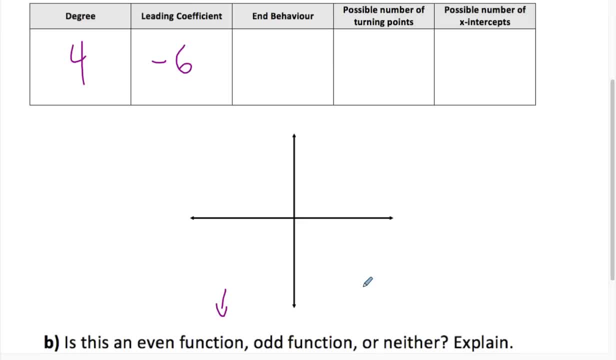 leading coefficient. That means it's going to go from quadrant 3 to quadrant 4.. What it does in between we don't really know for sure yet. I'm just going to make a rough sketch of an idea of what it might look like, But I know for sure it's going to start in 3 and finish in 4.. 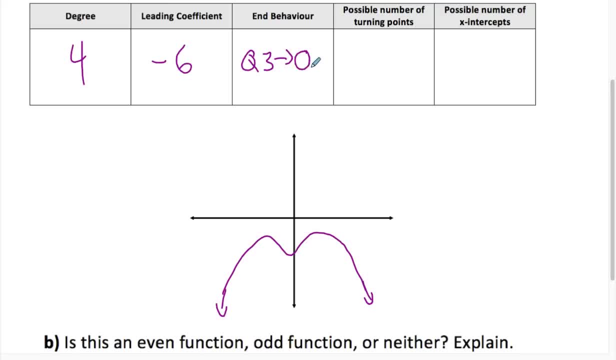 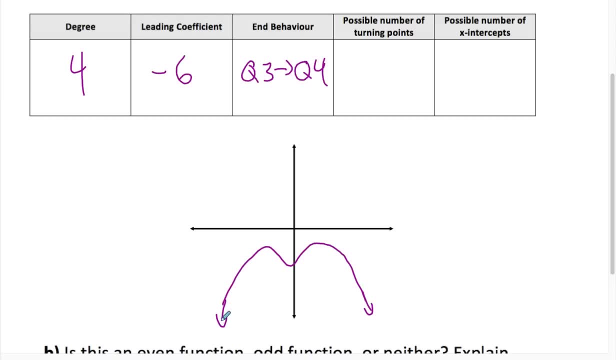 So end behavior: q3 to q4. Possible number of turning points. So if we have an even degree function it has to have the same end behavior. So if it starts going to negative infinity it has to finish going in the same direction. 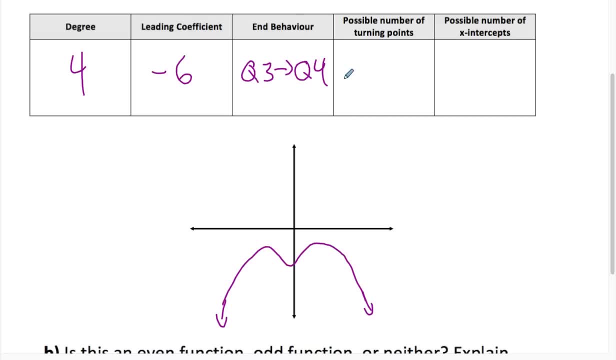 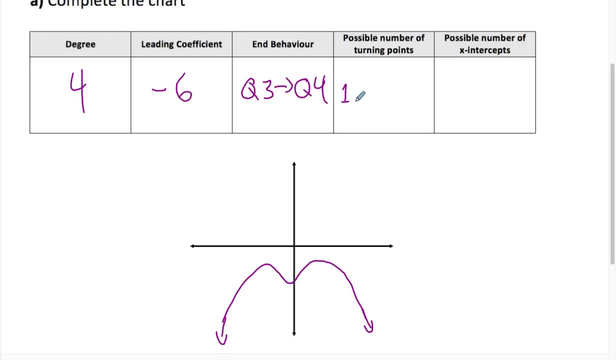 going to negative infinity. So it has to turn at least once And in order for it to finish going in the same direction, it could turn any number of odd number of times up to anything less than the degree of our polynomial. So it could turn once, or it could turn three times, like I've drawn: One, two. 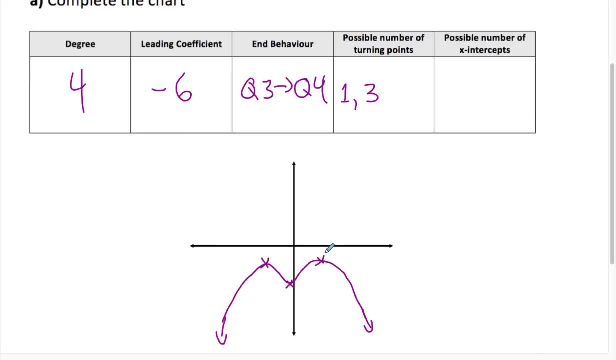 three, Three turning points, Or it could have just turned once like that, But I know for sure all even degree polynomials have an odd number of turning points. If I had an odd degree polynomial, so if it were to have opposite end behavior, something like this: it doesn't. 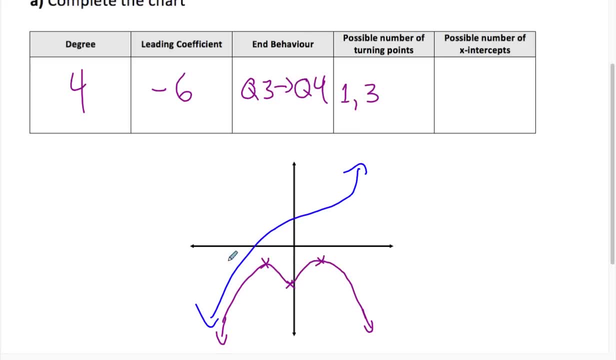 have to turn at all because it's going in opposite directions. And if it does turn it would have to turn back again, So it would have to have an even number of turning points. So: odd degree- polynomial: even number of turning points. even degree polynomial- odd degree number of. 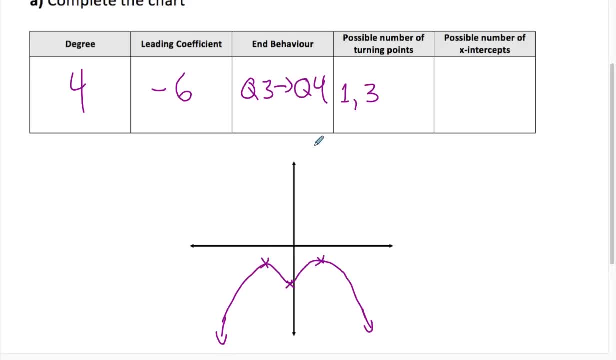 turning points. How about x-intercepts? Well, the one I've drawn doesn't even cross the x-axis, And that's valid for an even degree polynomial. So it could have zero or it could have any number up to and including the actual degree of your polynomial. 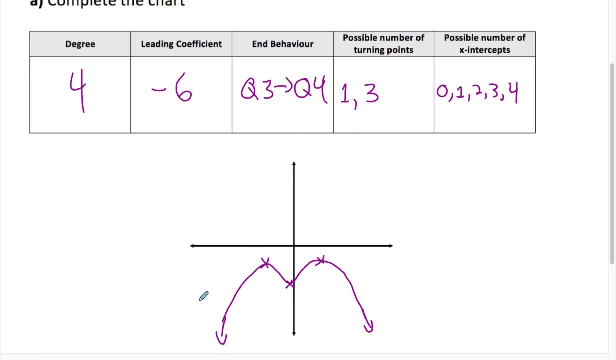 Now an odd degree polynomial. since it has to finish in the opposite direction, it has to at least cross the x-axis once. So if you have an odd degree polynomial, same rule, it could be anything, but it can't be zero. Let's look. 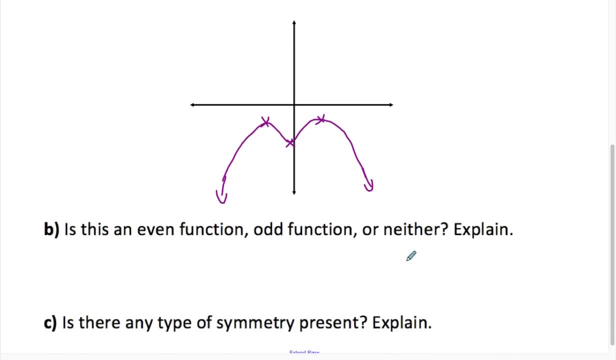 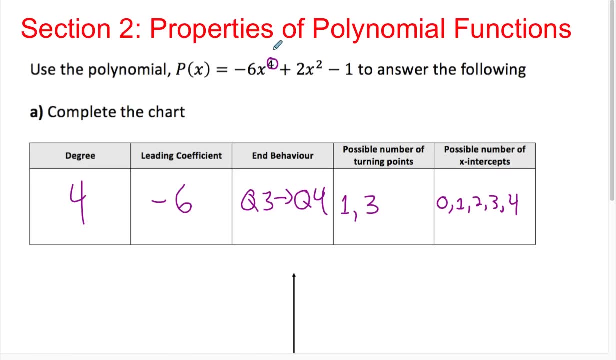 at stating whether this is an even function, odd function or neither. Well, we know it's an even degree function, but what makes it an even function is if each term is an even degree term. So this is degree four. that term's degree two. this term is: 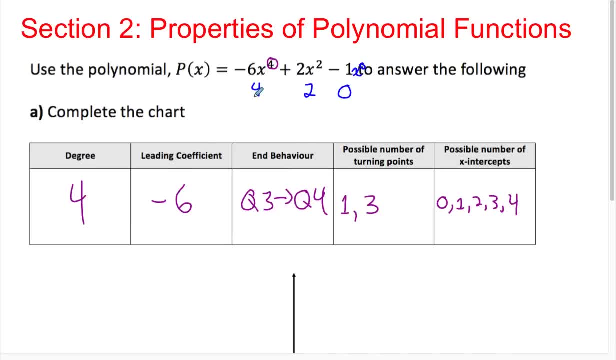 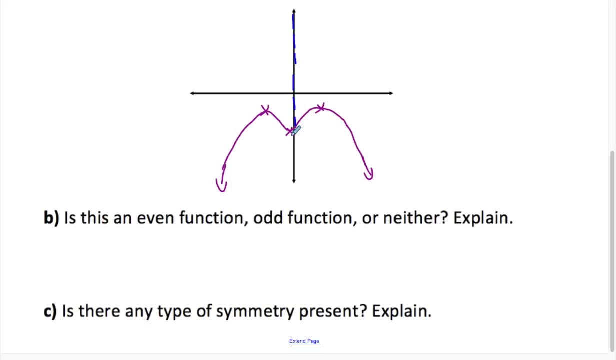 degree zero. right, It's an x to the zero. Since each of those is an even number, what we have is what we call an even function, which means it's going to have line symmetry right on top of the y-axis. So this is an even function. 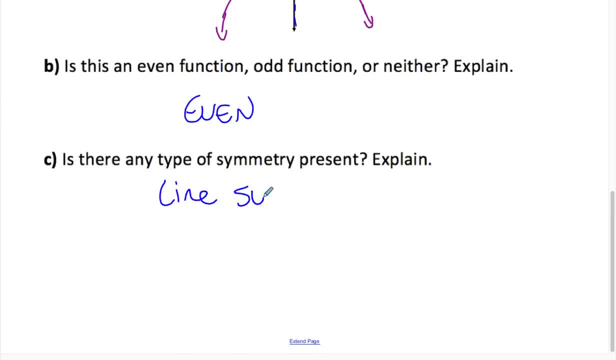 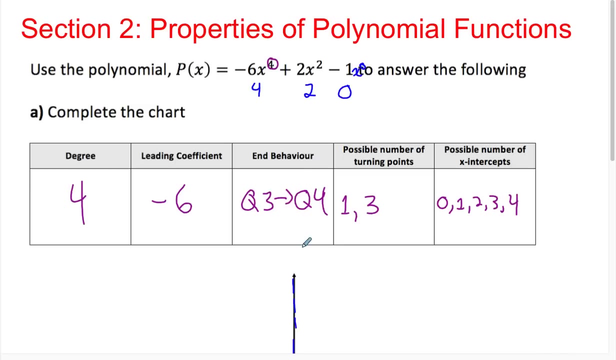 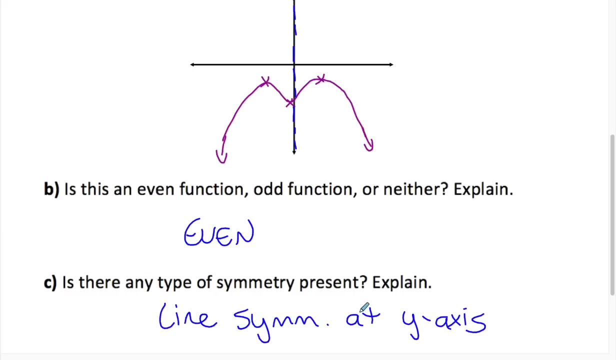 which means it has line symmetry at the y-axis. All even functions have this. What would make it an odd function is if each term was an odd degree term, and then it would have point symmetry at the origin. So one thing to keep in mind here is just because we have an even degree function doesn't mean that it is in fact an even function. 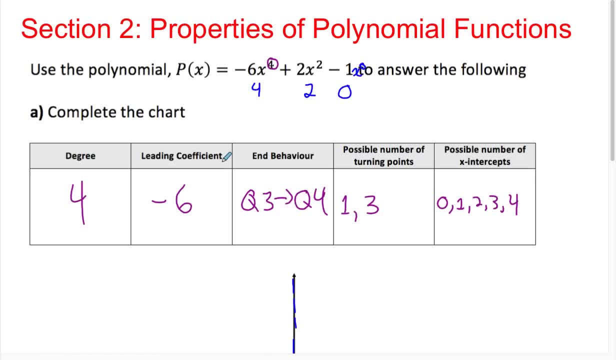 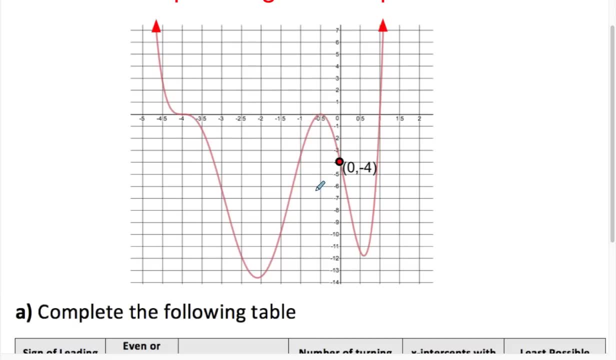 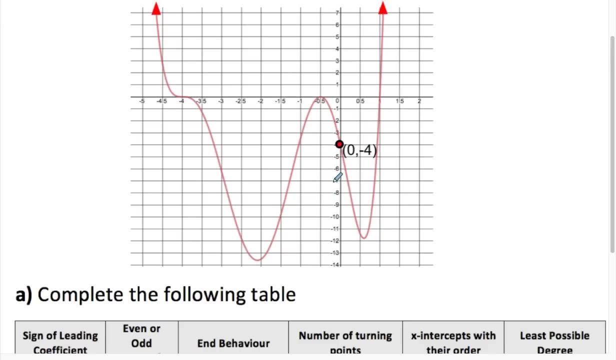 You have to make sure each term is even degree for it to be an even function. So let me give you the graph this time, and you come up with the equation for this exact function, given its graph. Before we do that, let's get some general properties of this graph. So we have 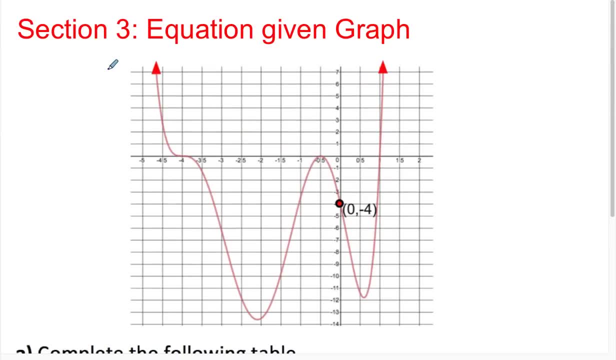 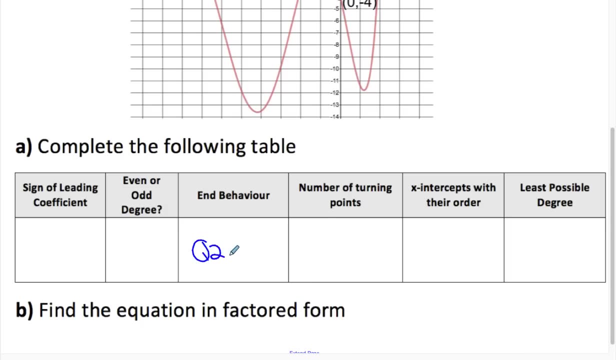 the same n behaviors here right. It goes off to positive infinity on the left, and it goes off to positive infinity when we go to the right And it goes from quadrant two to quadrant one, So n behaviors are q2 to q1.. Since it has the same n behavior, we know that it is. 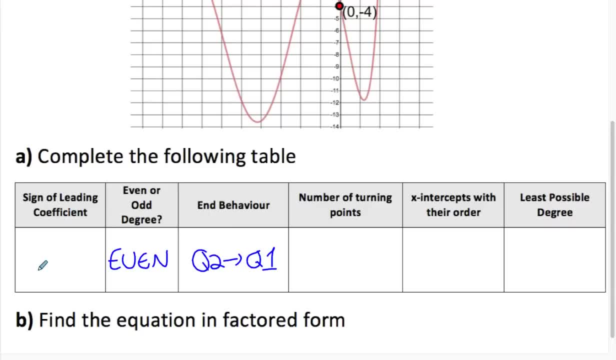 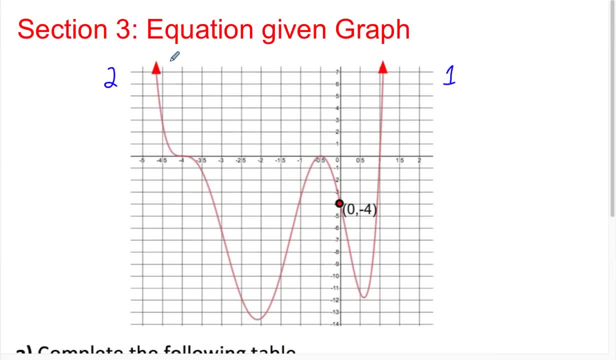 an even degree function. And since it goes from two to one, we know that the sign of the leading coefficient must be positive. Let's count the turning points. So where does the function change? from increasing to decreasing or vice versa? Right here, right here. 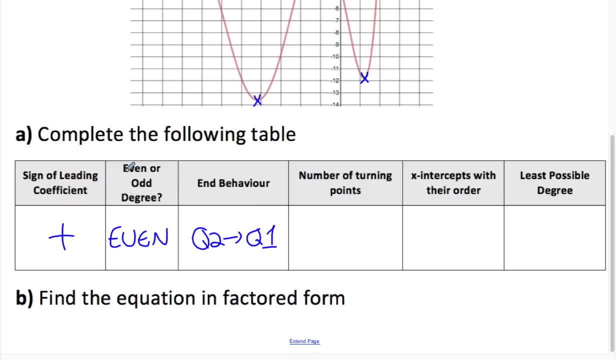 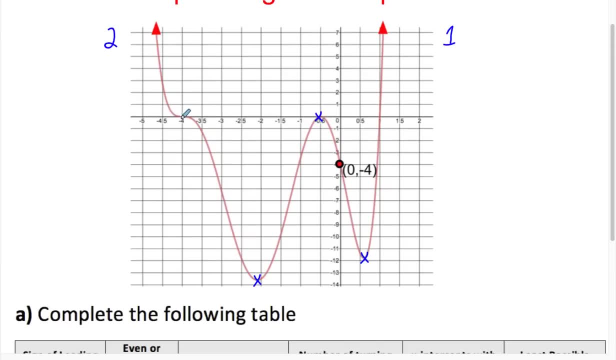 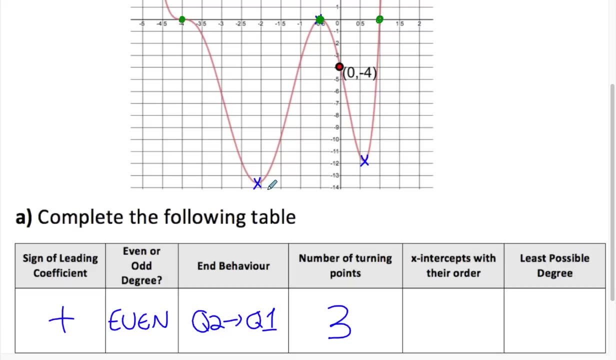 and right here I see three turning points. So number of turning points: Three: Let's find the x-intercepts. So we have x-intercepts here at negative four, here at negative a half and here at one. So let's write down those x-intercepts with their order And we can tell the order based. 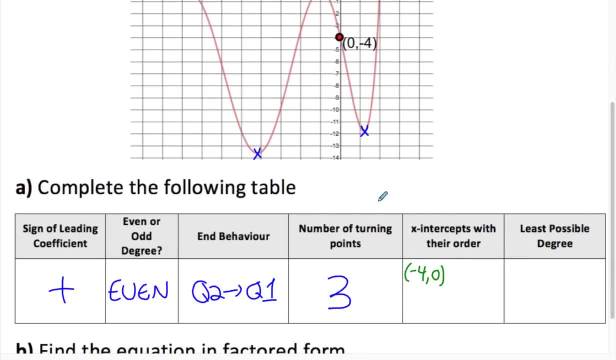 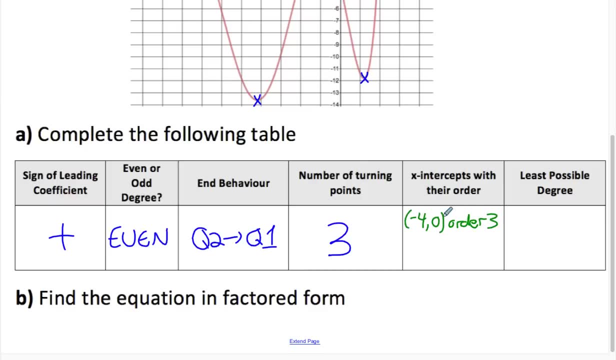 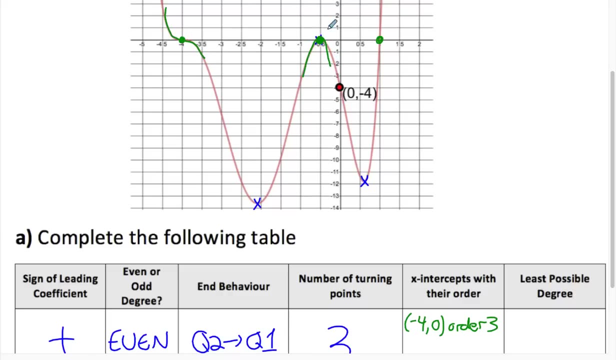 on the shape that it does at the x-intercept, So at negative four, zero. it makes this s shape, which means we have an order three root, Which means the corresponding factor is going to have an exponent of three on it, This one. it makes this parabolic shape where it just bounces off the x-axis, That's order two, So at 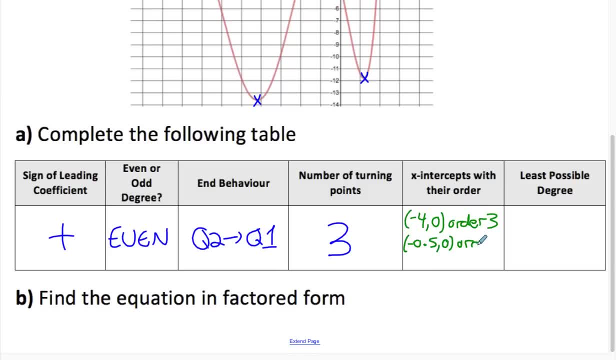 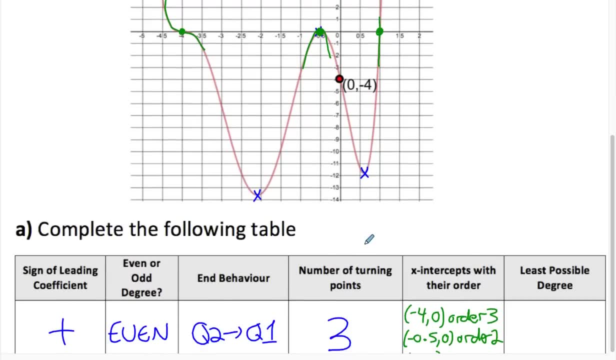 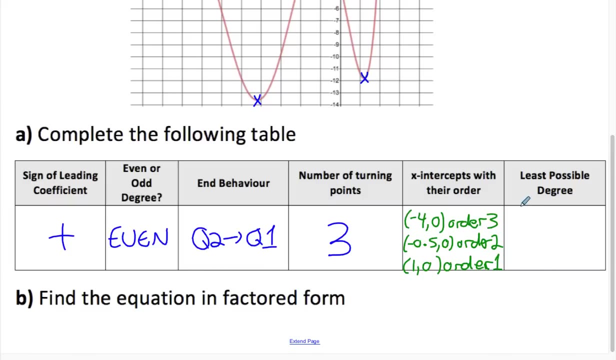 negative a half. we have an order two root And there was another x-intercept at one and I think that one just went straight through. So just straight through, so it just looks like a linear function. so it's just order one Least possible degree. So we can find that just by. 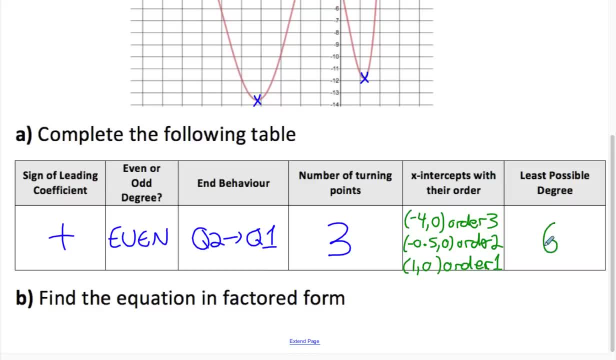 adding up the orders of our roots, So three plus two plus one six, And keep in mind a degree six, polynomial, it could have five, three or one turning points. It just so happens ours in this case has three turning points. Let's now find the exact equation for this. 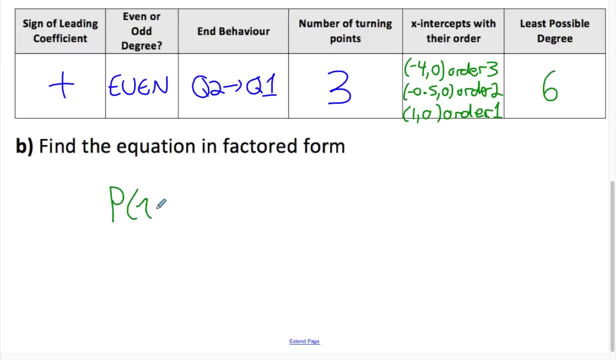 function. Now, this function- I'll just call it p- at x equals. so I'm going to write the equation in factored form So I can find its factors from its corresponding x-intercepts, from its zeros. So if x equals negative, four is one. 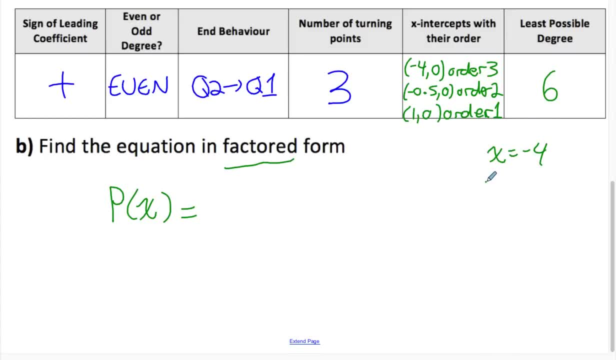 of the zeros to find the corresponding root. just rearrange this to set it to zero. x plus four equals zero. must have been the corresponding root. So x plus four is a factor of this polynomial function And it's order three, which means the exponent on this factor. 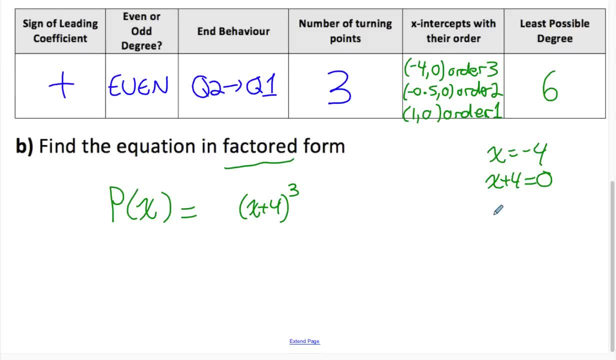 must be three. Now x equals negative. a half is also a zero of this function. Rearrange this. setting it to zero, I get two x equals negative one. So two x plus one is a corresponding factor. So two x plus one is a factor with an exponent of two. And similarly, if x 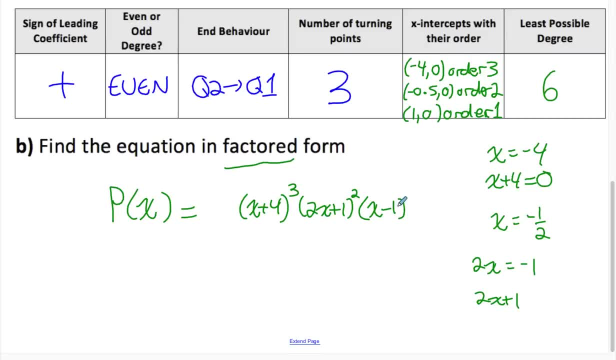 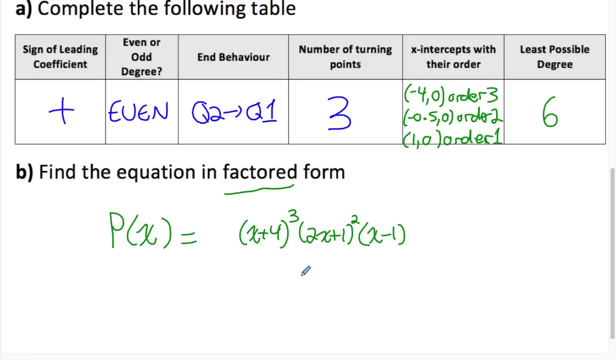 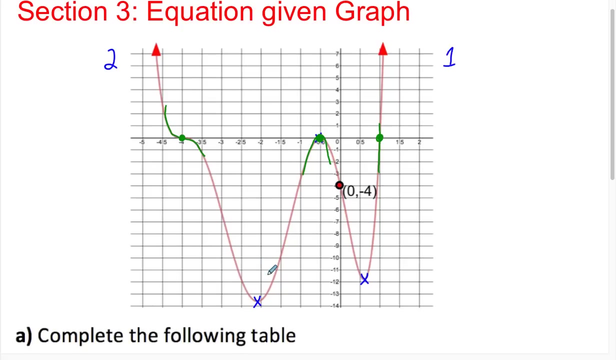 equals one is a zero. that means x minus one is the corresponding factor exponent of one. This is the equation of the family of polynomial functions that would have these x-intercepts. I'm going to have to put this variable k here as well. So this is the equation of the family of functions that has those corresponding. 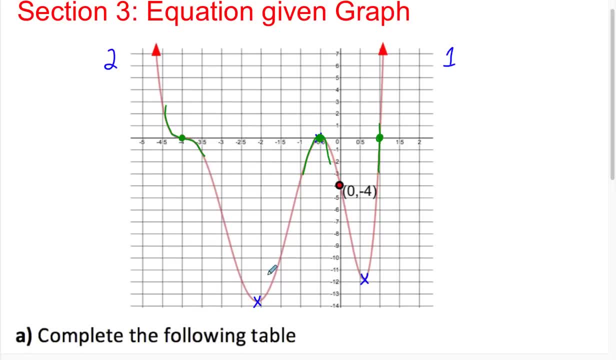 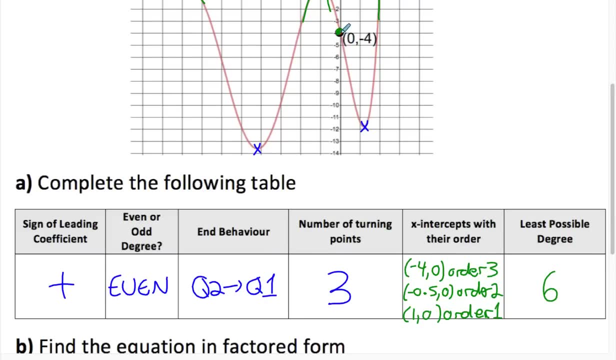 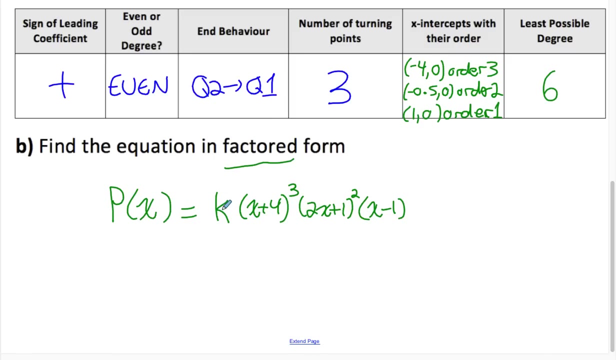 x-intercepts with those orders Attached to their roots. If I want this specific member of the family that passes through this exact point, I'm going to have to solve for this value of k that is going to tell me this one specific member of the family. Like I could draw an infinite number of polynomials. 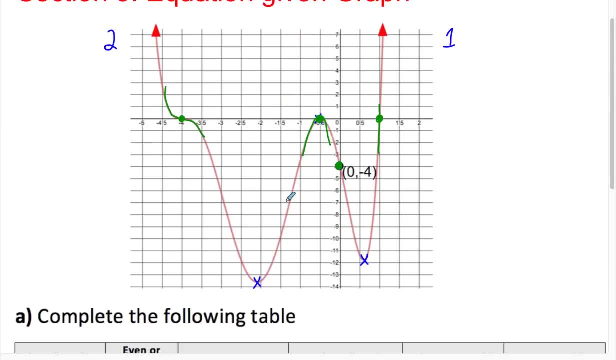 that have these exact roots. But if I want the one that is stretched in this exact way, that goes to this exact point, I will have to sub in for x and y and solve for k. So let's do that, So I'll plug in. so remember: p at x means the y value. so if I 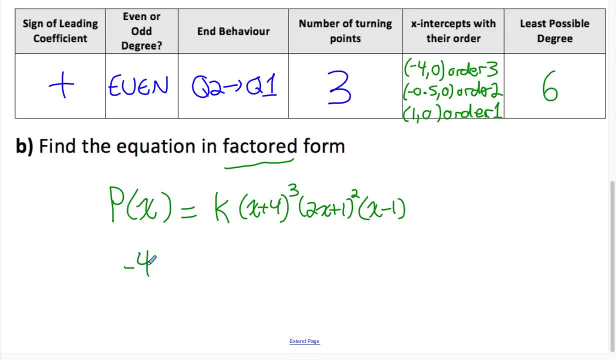 know p at zero equals negative four, so I can plug in zero for all the x's. and then I know p at zero will be negative four equals k zero plus four, cubed two times zero plus one, squared times zero minus one. 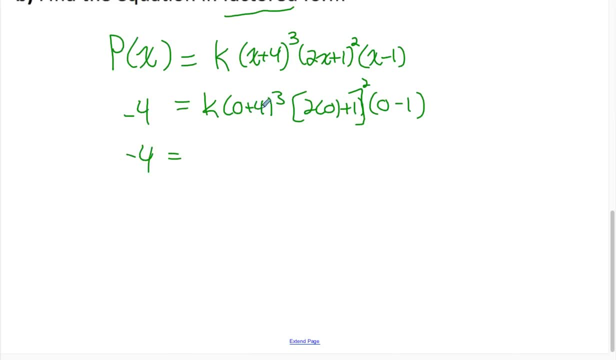 And I'm not going to spend much time solving this, I'll just do it very quickly. Zero plus four is four. four cubed is sixty-four, So I've got k sixty-four. two times zero is zero. plus one is one. one squared is one. so times one, times negative one: 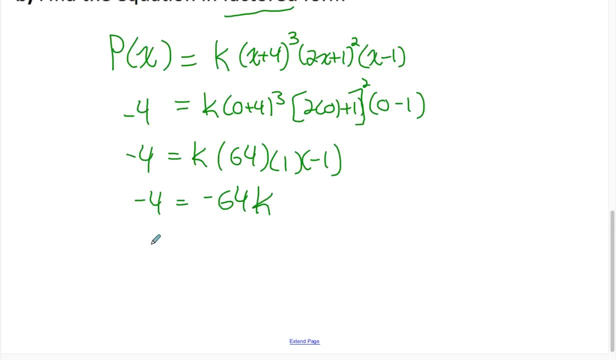 So negative four equals negative sixty-four. k Rearrange k equals negative four over negative sixty-four, that's one over sixteen. So if I want the specific equation for this member of the family of polynomial functions, I have to put one over sixteen in front of all the roots. So p at x equals one over sixteen. 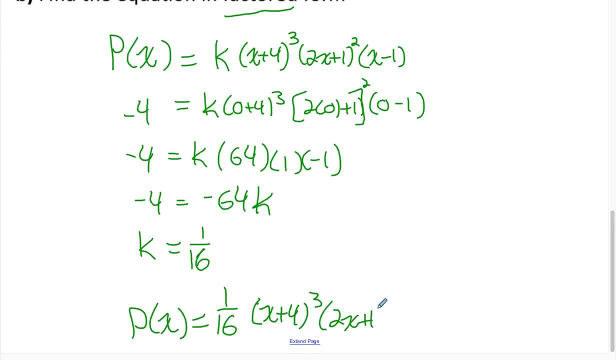 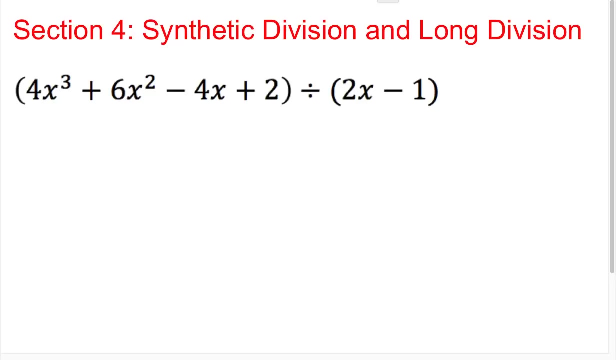 and then all of the corresponding roots with their proper orders. There we go. There is the equation of this graph. Next, let's look at how to divide polynomial functions, and this will lead us into being able to factor and solve different polynomial functions. 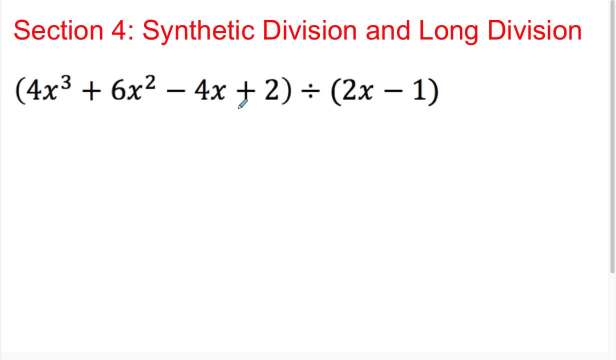 So you would have learned two methods. probably in your course You would have learned synthetic and long division. So if you're dividing by a linear divisor, so this is a linear divisor. right, it's degree one If the coefficient of the linear divisor is not one. 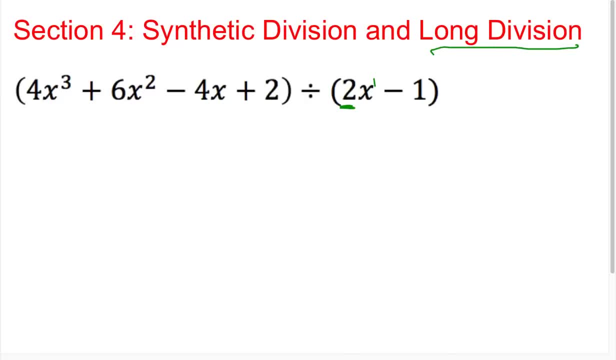 so in this case it's two. I recommend using long division. I think that's easier If you have a linear divisor. so degree one, where the coefficient is one, I recommend doing synthetic division. It's a lot quicker. So let's practice both of those. 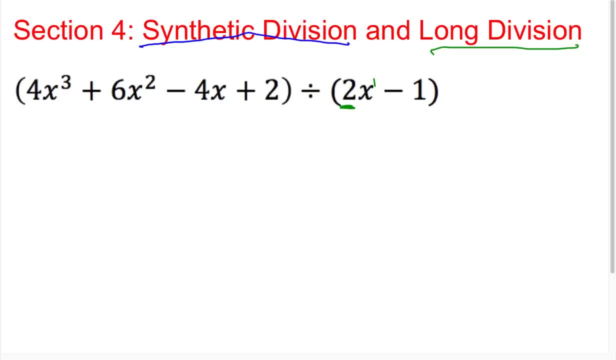 So long division. you start by writing your divisor here, so two x minus one, and then we will write our dividend, making sure that all degree terms are represented. We have degree three, two, one and zero, So we don't have to worry about filling any zero terms in. So four x cubed. 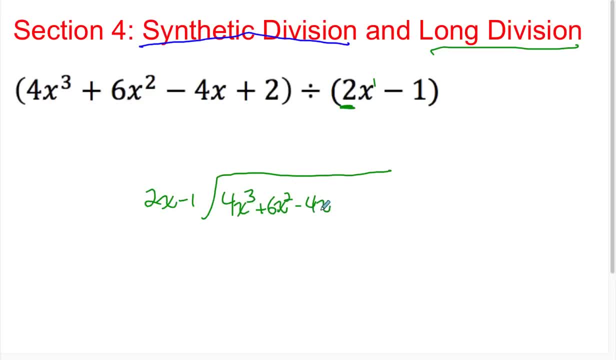 plus six, x squared minus four, x plus two. And then what you're going to do is you're going to follow for long division. we follow the steps: divide, multiply, subtract, repeat, Divide, multiply, subtract, repeat, Divide, multiply, subtract, repeat, And you just keep going. 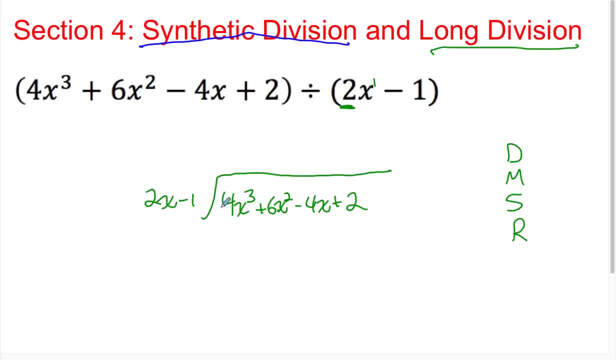 until you're finished, until you have your remainder. So we start by doing the highest degree term and the dividend: four x cubed divided by the highest degree term in the divisor two x. So four x cubed divided by two x gives us two x squared, And what you need to do is you need to write that above its. 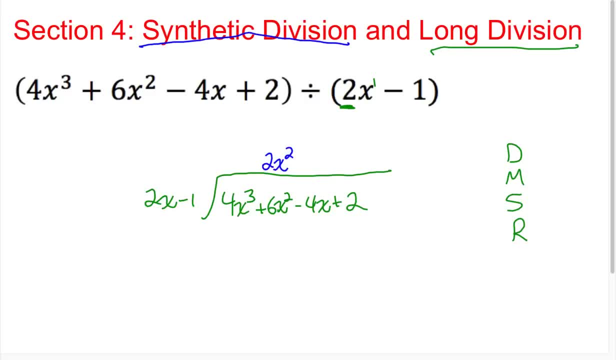 like term. So two x squared is degree two. so write it above the degree two term in the dividend. Now we multiply, So we did divide. now we multiply. We multiply this number in our quotient by both terms in the divisor. So two x squared multiplied by two x and negative one. 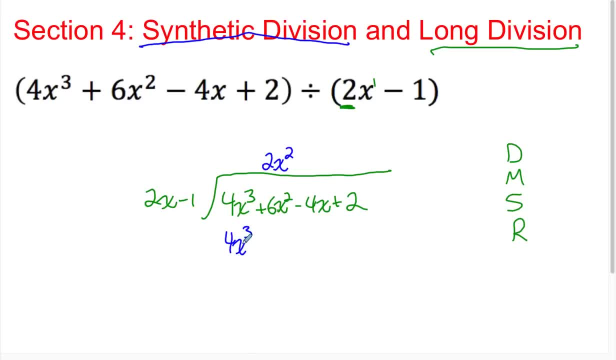 So two x squared times two x is four x cubed. Line it up with its like term: Two x squared times negative, one negative two x. Line it up with its like term And then we subtract. So we subtract the like terms: Four x cubed. 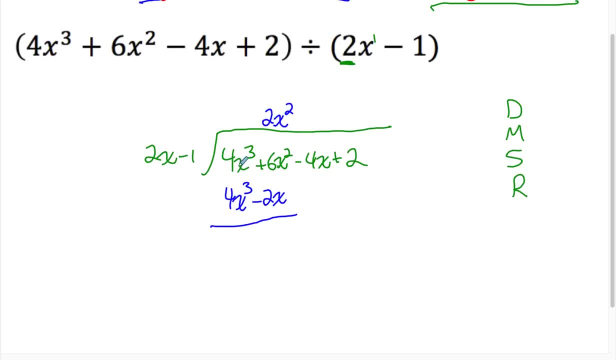 minus four x cubed is zero x cubed. That's what we want. That shows us we're on the right track. Six x squared minus negative. two x squared- Sorry, I forgot my squared earlier. Two x squared times negative. one is negative. two x squared Subtract Six. 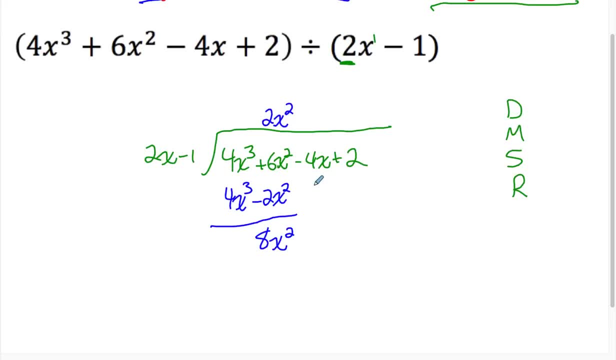 minus negative two is eight x squared. And then we bring down our next term minus four x. And then we repeat, So we divide it, multiply, subtract. Now we repeat, So we do, the first term in our dividend, So eight x squared divided by our first term in our divisor. So eight x squared divided by two x. 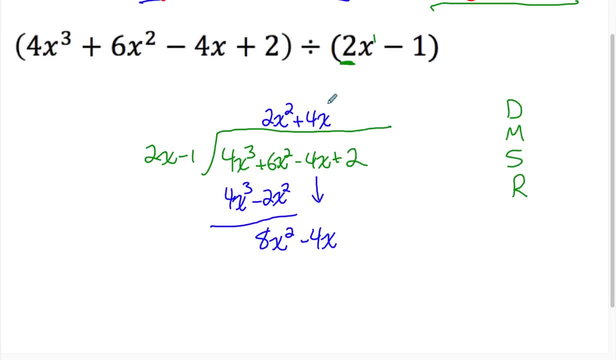 is positive four x. Then we multiply Four x multiplied by two x minus one. So four x times two x is eight x squared. Line it up with its like term: Four x times negative one. negative four x. Now we subtract So negative four x. take away negative four x, That is. 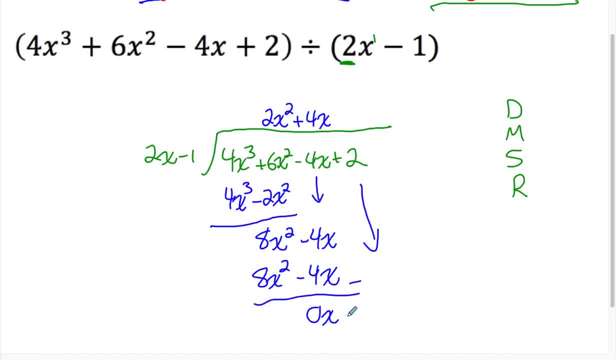 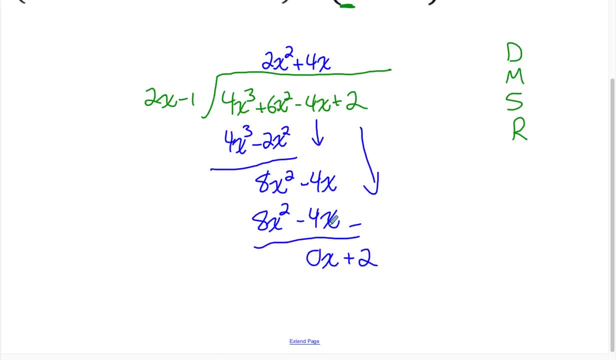 zero x, Then we bring down our next term positive two, And then we repeat. So when it's zero x, I guess you don't really have to repeat. Two is just going to be our remainder, But I'll just show you how the process finishes, for when this doesn't turn out to 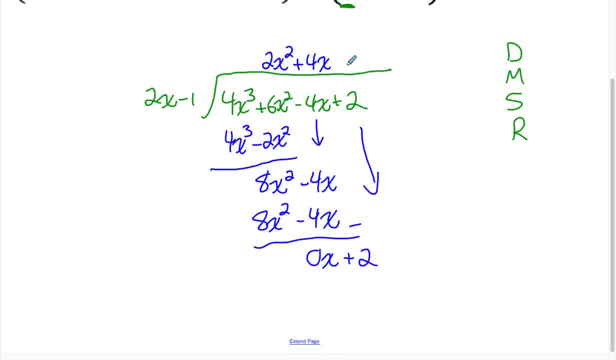 be a zero x as well. So we would do zero x divided by two x, That is zero. And then we multiply Zero times two. x is zero x. Zero times negative one is zero. Subtract Two minus zero is two. We have nothing else. 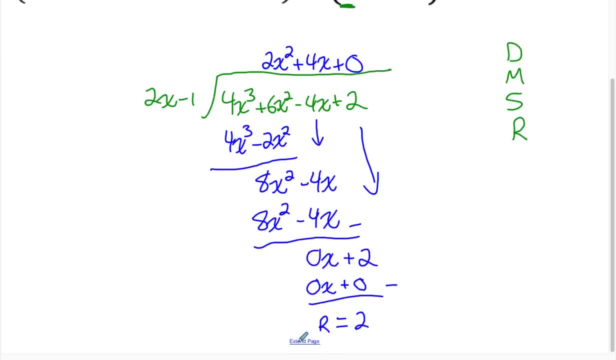 to bring down. So that's our remainder, And we can write our answer in two different forms. We can write it in quotient form. So we can write down: our dividend over our divisor equals our quotient. So four x cubed plus six x squared. 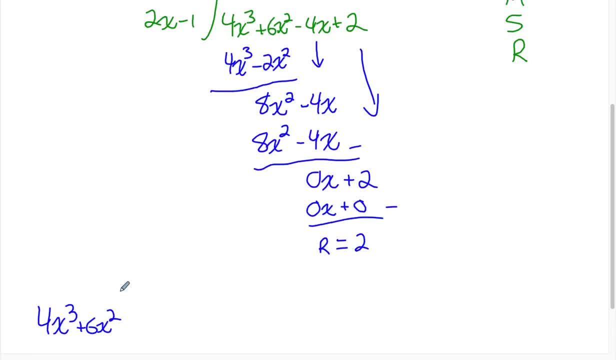 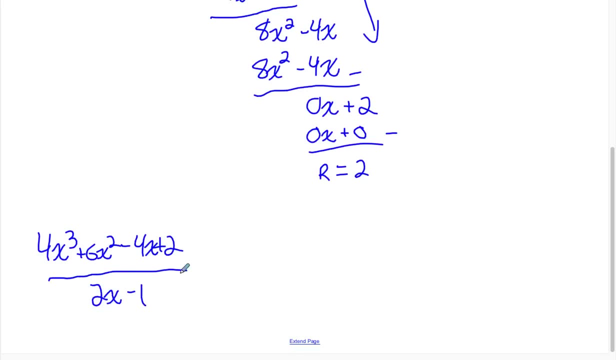 Minus four x plus two, Over our divisor Two x minus one. So this is the division we did. Equals our quotient Two x squared plus four x. Two x squared plus four x. No point in writing. the zero Plus the remainder. 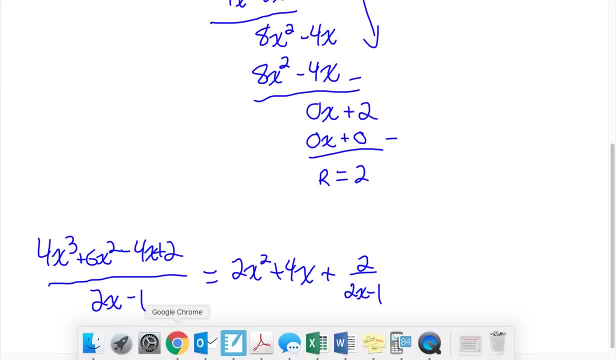 over the divisor. So that's what we call quotient form. I'll write my next answer to the next division using the multiplication statement so that you see both ways to write your answer to a division. So this is what we call quotient form. So dividend over divisor equals quotient plus remainder over. 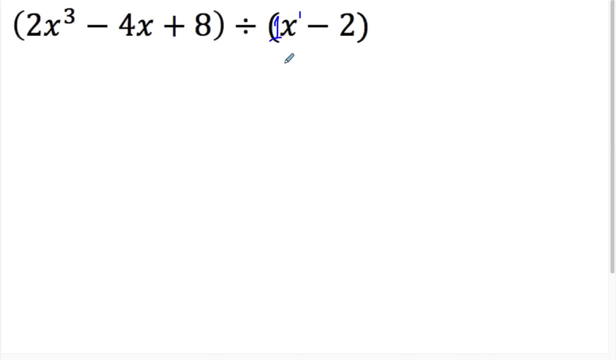 divisor. That's how that works. Now let's divide by a linear divisor that has a leading coefficient. that's just one. So we could use synthetic division. So we set up a chart like this And what we do is we put the zero of the divisor. So the zero. 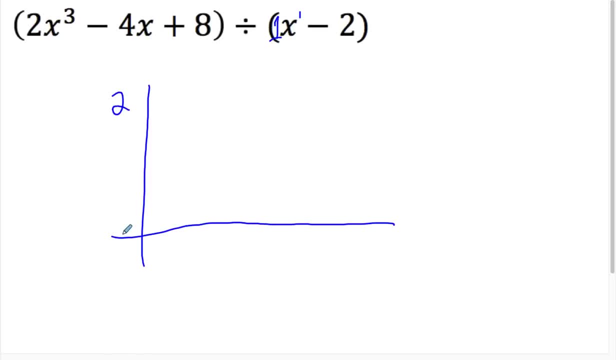 of x minus two. If we were to set that to zero and solve, we would get two. We put that here And then we write the coefficients of each term in the dividend up here. So keep in mind this one is missing a degree two term, So the degree three term, the coefficient. 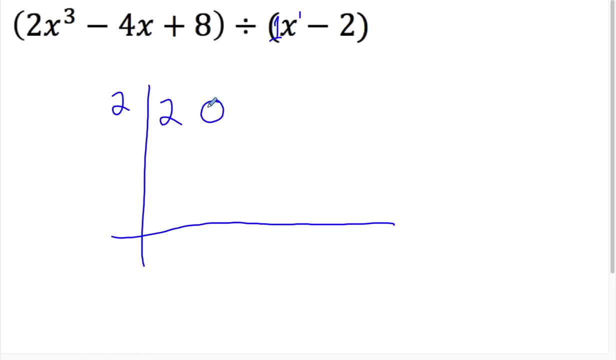 is two. The degree two term isn't there, so it must have a coefficient of zero. We have to include that The degree one term coefficient of negative. four. The degree zero term coefficient of eight. So what we're going to do is we're going to put a multiplication sign here and an addition. 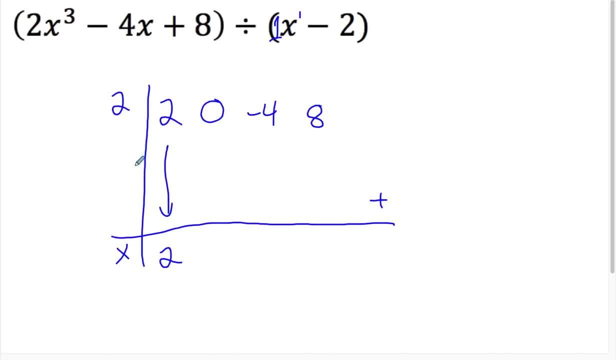 sign here. And here's how synthetic division works. You bring down the first term, Then you do your zero multiplied by this number. So two times two is four, So you put four here. Add Zero plus four is four, Then you do two times four, That's eight. So I brought that product up there. 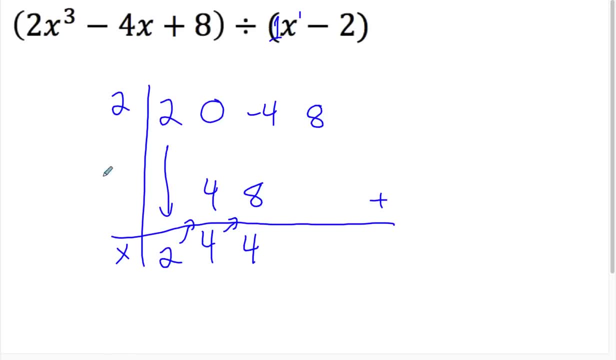 Then you do negative. four plus eight, That's four. Then two times four, That's eight. Then eight plus eight, That's sixteen. So these numbers tell us about our quotient. This is our remainder. This is the constant value. This is x. This is x squared. 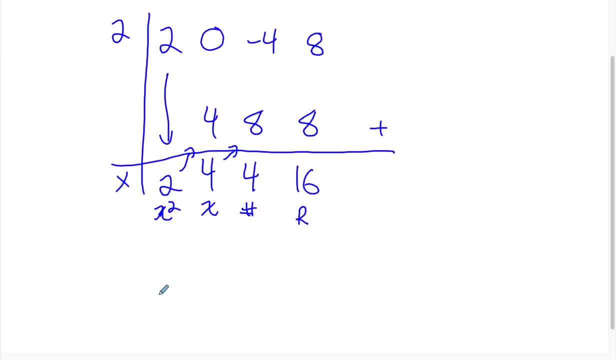 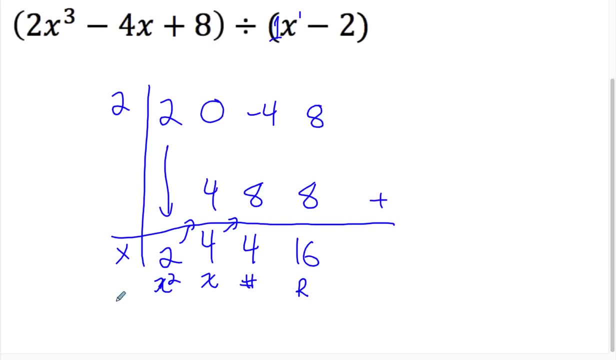 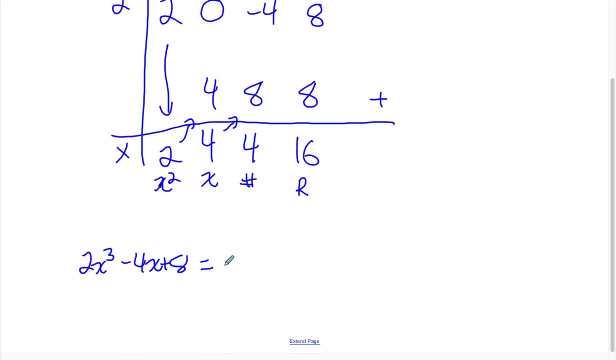 And I'm going to write my answer using the multiplication statement that I could use to check the division. So this dividend here, two x cubed minus four x plus eight, Two x cubed minus four x plus eight, is equal to the divisor which was x minus two. 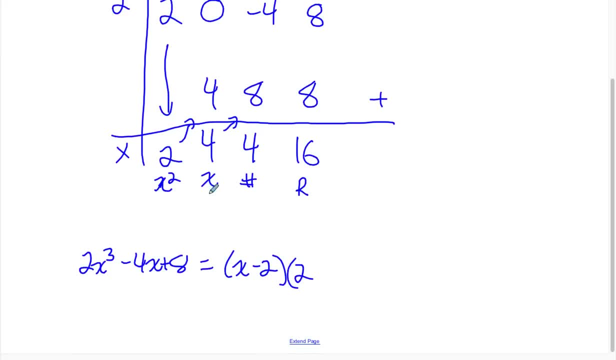 multiplied by the quotient which is two x squared plus four x plus four. So two x squared plus four, x plus four plus the remainder of sixteen. So this is the multiplication statement that you could actually use to check and make sure you did your division properly. You could expand this and collect. 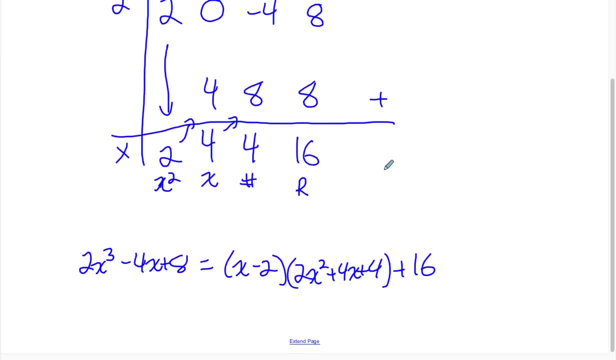 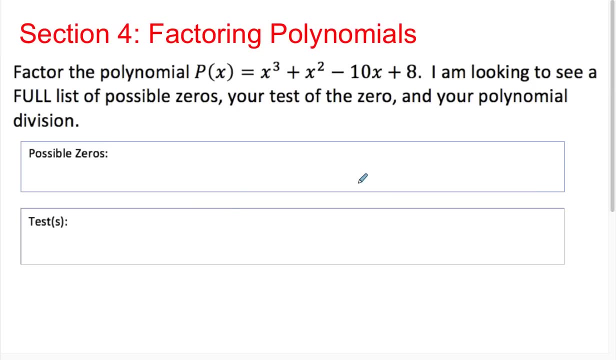 and you should get equal to your original dividend. Next, let's look at how to actually factor a polynomial. So this time I'm not going to tell you what to divide it by, But what we want to do is figure out how we could factor a polynomial. 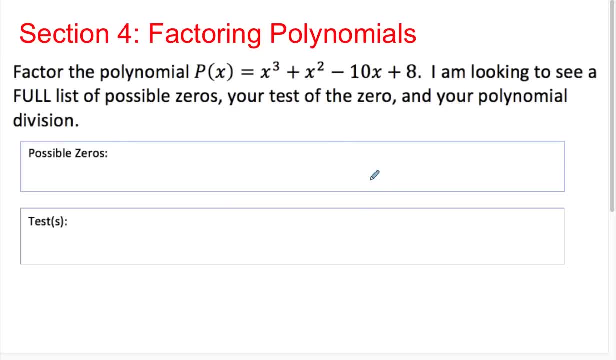 That's higher than degree two. So I have a degree three, polynomial. I first want to figure out what is going to divide evenly into this function. So what, when I divide it by its corresponding zero, am I going to get a remainder of zero? And it turns out there's the possible things that are going to be zeros of this function. 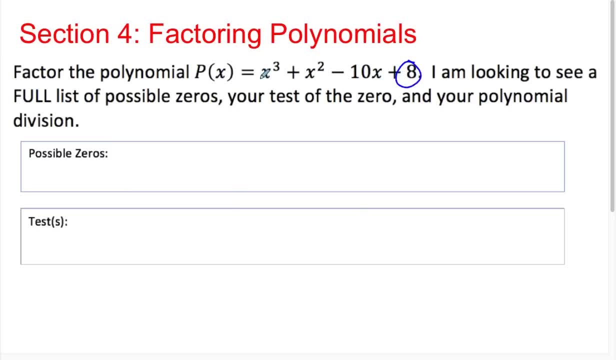 are going to be factors of your constant term divided by factors, the leading coefficient, But this time it's just one, So we can just look at factors of the constant term. So factors of eight are plus or minus one, two, four and eight. So these are the only possible numbers that could be zeros of this polynomial function. 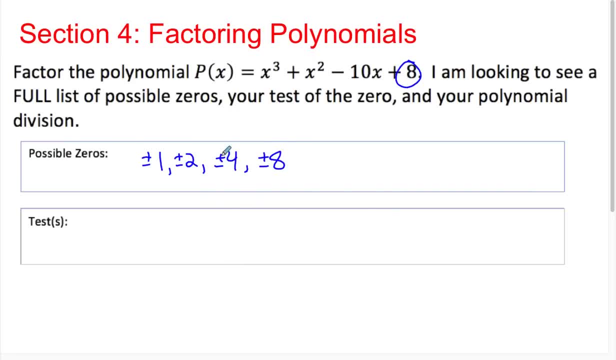 So that means, if I were to, what I need to do now is figure out which- well, there's going to be more than one that works, But let's find one that works. So then, when I know, so then, when I divide by its corresponding root, I'll get a remainder of zero, And what I'll have done is I will have 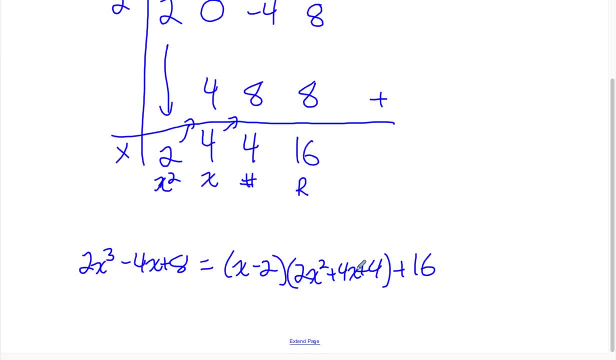 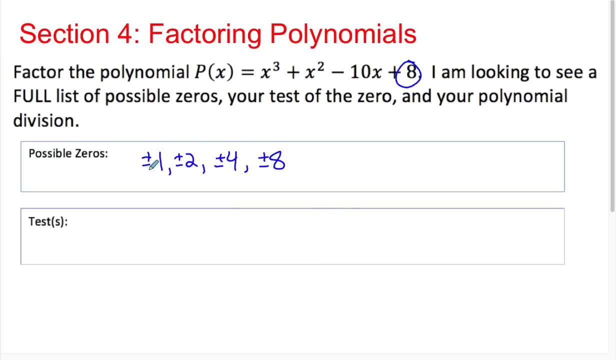 factored the original polynomial into two factors like this, and it won't have a remainder as long as we divide by a root, that is a zero of the function. So you would test a bunch of these. So if we tested p at one, we would do one cubed plus one squared. 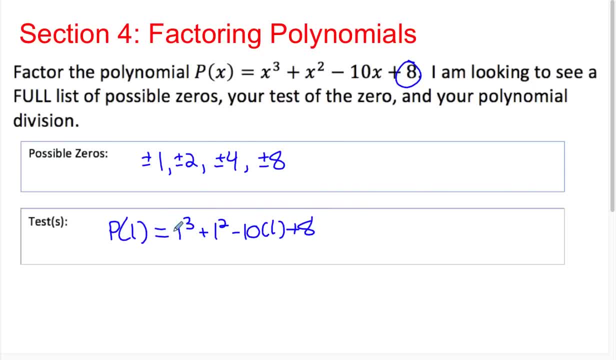 minus ten times one plus eight. So we have: one plus one is two minus ten is negative. eight plus eight is zero. So since p at one is zero, that means the corresponding root x minus one must be a factor, if is a factor, of our original polynomial. So that means, if we divide this original polynomial by 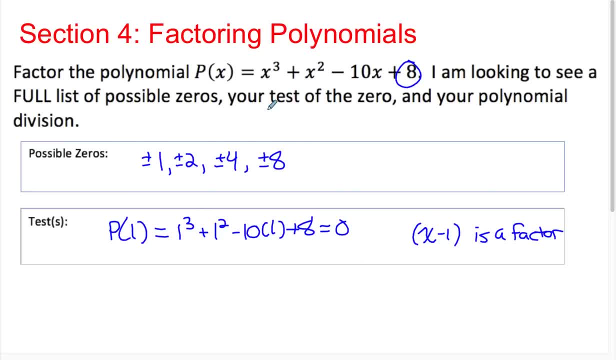 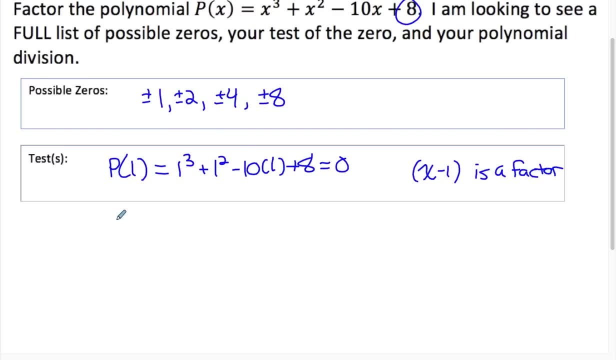 x minus one, we will get no remainder, and that's what we want. to factor a polynomial. So let's divide x cubed plus x squared minus ten, x plus eight by x minus one, and I'll just do it using synthetic division very quickly, since we've already reviewed that. So the zero is one. put that here. 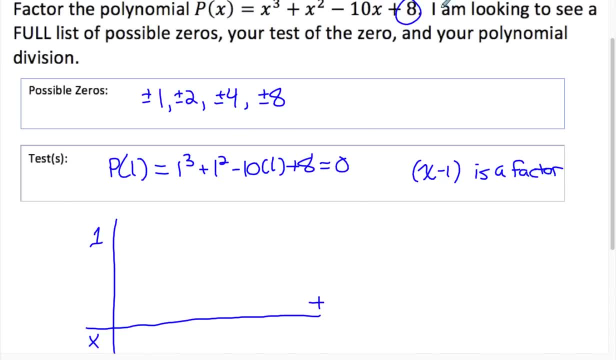 multiply, add and put all the coefficients of the terms and it's not missing any terms. So just one. one. negative ten: eight. quickly bring the one down: One times one is one. One plus one is two. One times two is two. Negative ten plus two is negative eight. One times negative eight is: 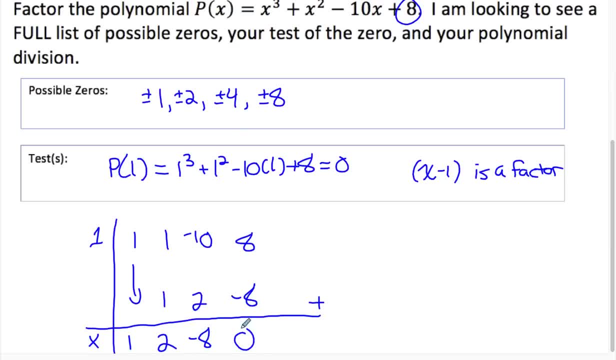 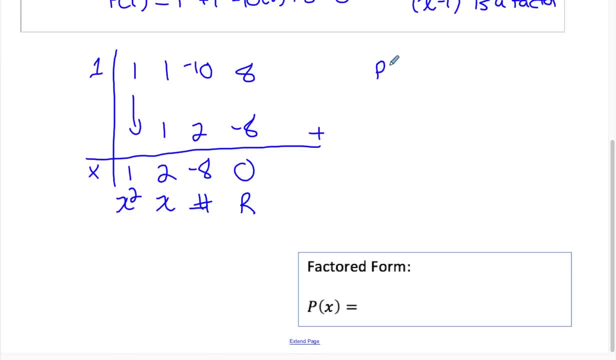 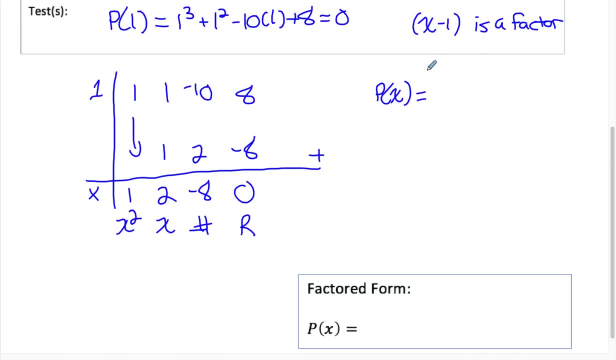 negative eight. Eight plus negative eight is zero. So what we have found is that no remainder. This is our constant term. This is x. This is x squared, So p at x is equal to. So this polynomial function is equal to the root that I divided by x minus one. 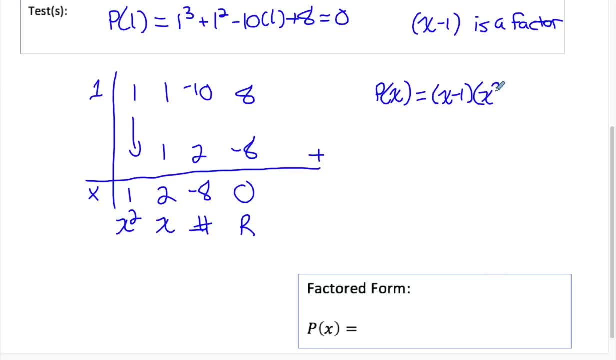 multiplied by the quotient x squared plus two, x minus eight, And then we check: can we factor this any further? So I have a quadratic here that I can factor just by finding the correct product and sum. So multiplies to negative eight, adds to two is four and negative two, So this factors to x minus one. 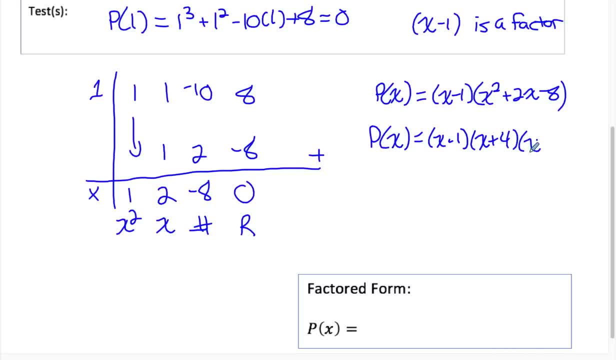 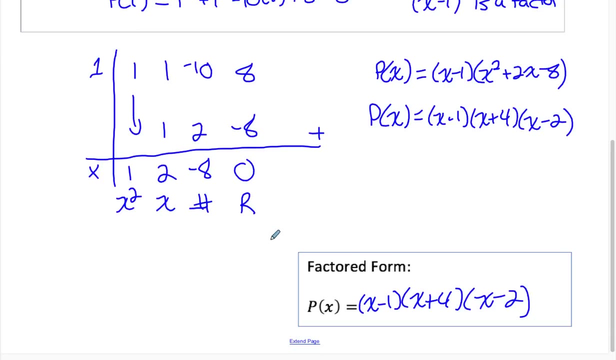 x plus four, x minus two. So my factored form of this polynomial: x minus one, x plus four, x minus two. If I were to expand this all out I would get back to my original polynomial. but having in factored form is good, because then I can see all. 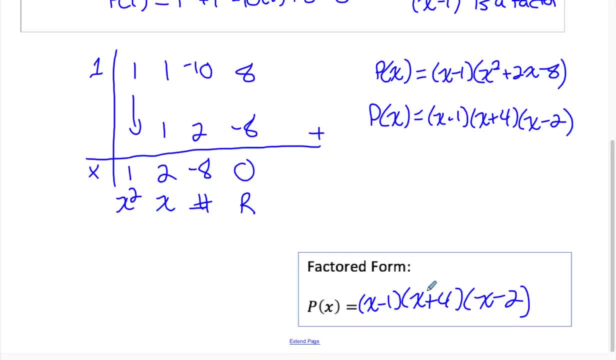 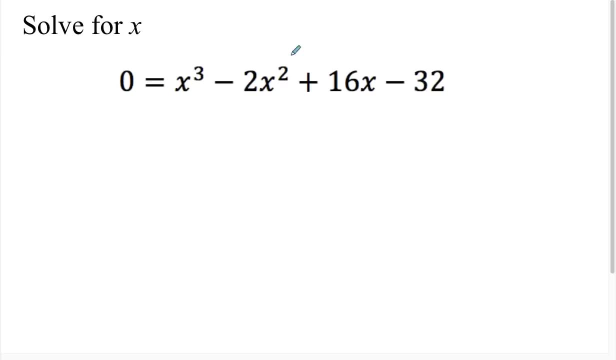 the x intercepts One, two negative four, and I can get a more accurate graph of this polynomial. Let's solve this function. So, if I want to solve this function, it's already set to zero, So I'm going to. in order to solve it, I'm going to have to get it into a form. 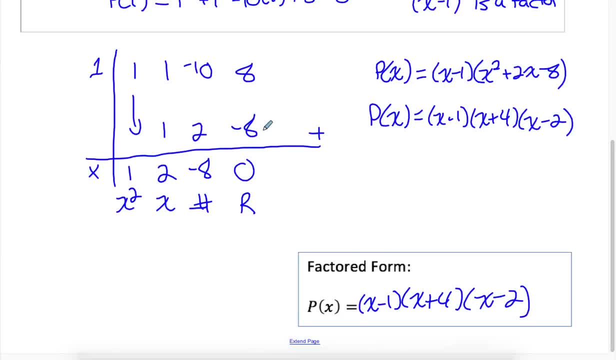 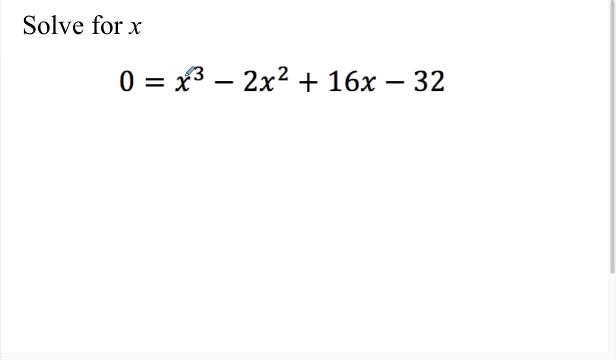 like this. I'm going to have to get it into factored form. Once you have it into factored form, you can use the zero product rule, set each factor to zero and solve. So if I want to factor this, I have two options here. I could test factors of negative thirty. 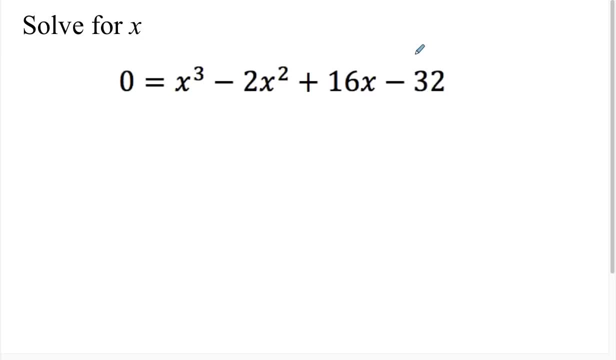 two, find a zero and then use synthetic or long division. but it might be helpful for you to check and see if you can do a factoring by grouping shortcut, because sometimes that works. So if I were to group the first two terms together: x cubed minus two, x squared. 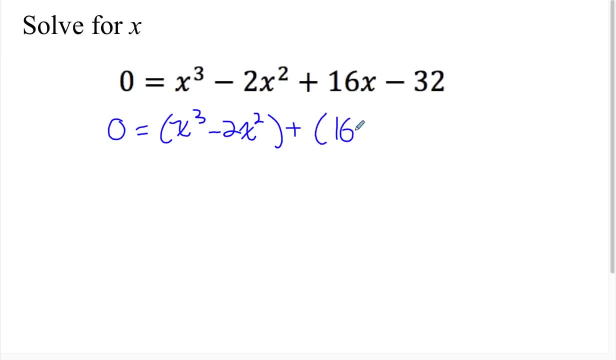 and if I were to group the last two terms together, sixteen x minus thirty two? and then if I were to common factor each group separately, check and see if you get a common binomial. So from the first group I can common factor out an x squared divide. 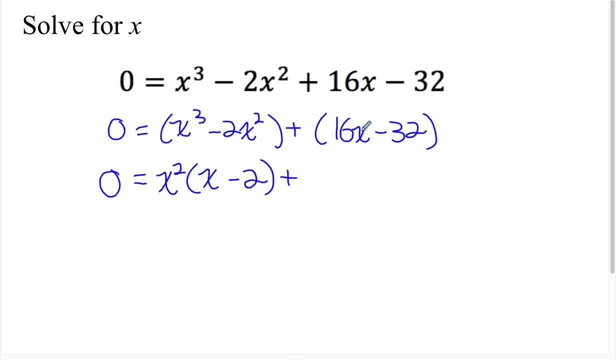 them both. by what I took out, I would get x minus two. Second group: I could common factor a sixteen, divide them both by the sixteen I took out and once again I would get x minus two. I get this common binomial. So factoring by grouping works. What I could do now is common. 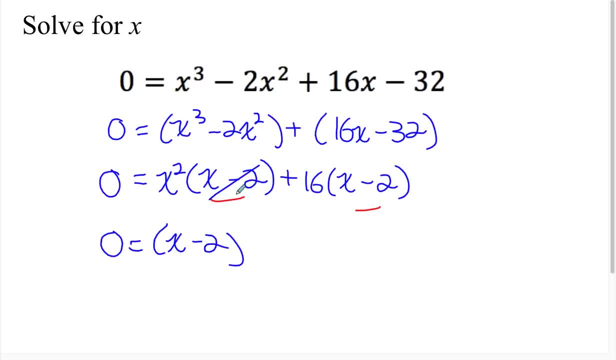 factor out that common binomial from both terms and what I'm left with is x squared plus sixteen as my second factor. So I've now fully factored this. so zero product rule. if the product of two things is going to be zero, either that one. 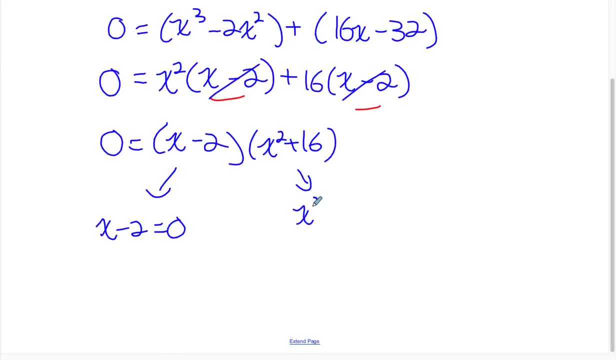 has to be zero or this one has to be zero. So, after you've fully factored it, set each factor to zero and solve each factor, So solving this equation. I would get x equals two. If I tried to solve this equation, x squared equals negative. 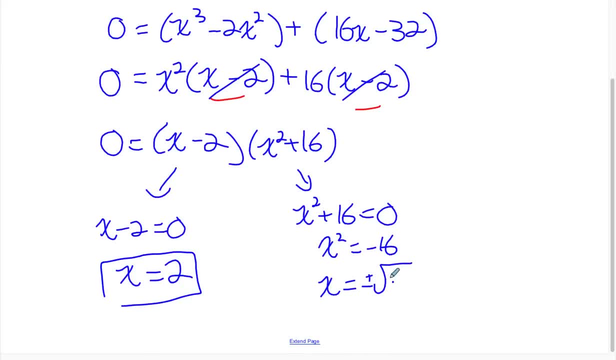 sixteen. x equals plus or minus root negative sixteen. we can't square root a negative. no solutions for that factor. So my only answer that would make this original polynomial equal to zero would be an x value of two, and whenever you're solving an equation you can go back and check and make sure you did. 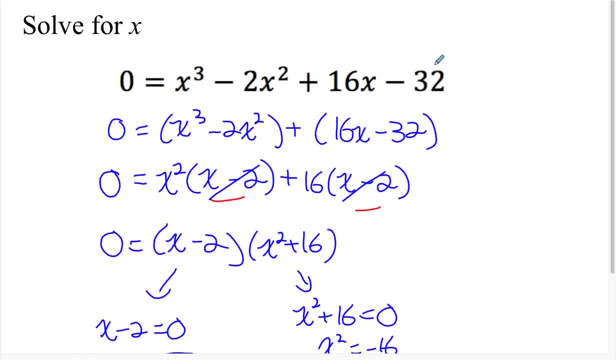 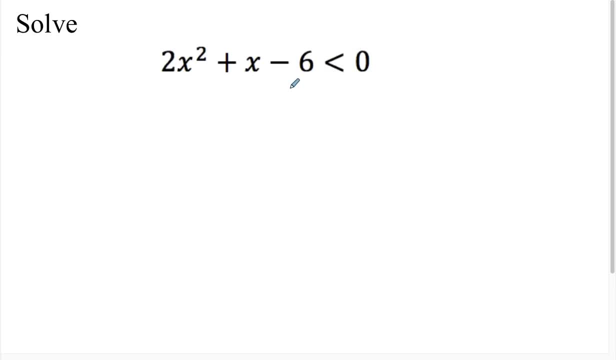 it properly. Sub two back into the original equation, make sure it equals zero. How about if we have an inequality? So we don't want to know what value of x makes it equal to zero, We want to know what value of x or what range of values of x is will make this function. 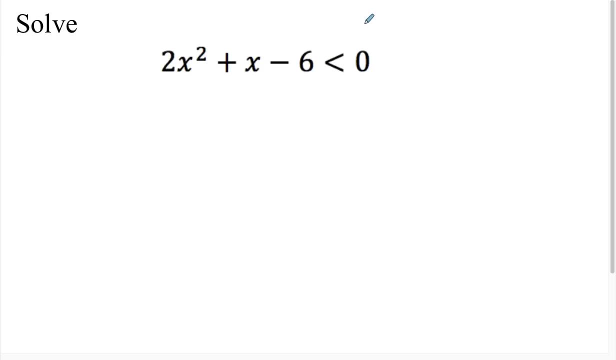 be less than zero. So we have two options here: We can make a factor table or, if the function is easily graphed, we could just get a rough sketch of the graph of the function and go from there. So for this function, since it's just a quadratic, I would just do a rough sketch. 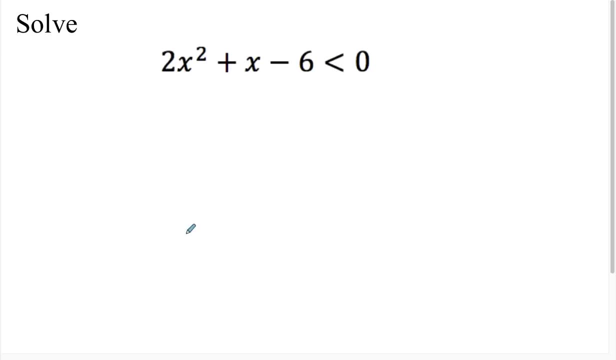 of this graph and answer the inequality from there. So if we want to graph it, it's useful to put the polynomial into factored form. So if we want to factor this polynomial, I would need to find two things that have a product of a times c, so negative twelve. 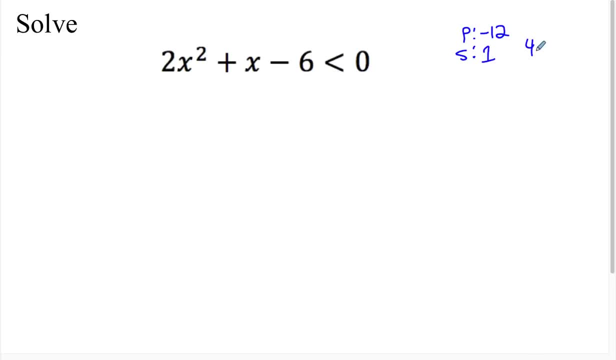 and a sum of b, which is one, And those two numbers are four and negative three. So hopefully you know how to factor a polynomial where the leading coefficient is not one. You know you break up the middle two terms into the numbers that satisfy your product and sum. 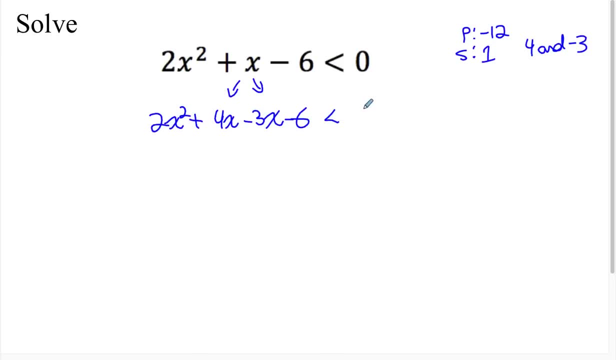 Leave the first term and last term and then you factor it by grouping So factor. common factor from the first two terms: two x, x plus two. Common factor from the last two terms: take out a negative three gives us an x plus two as well. 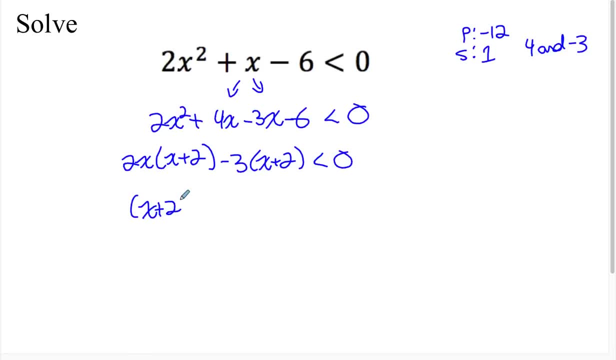 And then you have a common binomial, So x plus two, two x minus three. So my zeros, my x intercepts, my x intercepts of this function are going to be at negative two, zero. And if I were to set this to zero and solve, I'd get three over two, which is 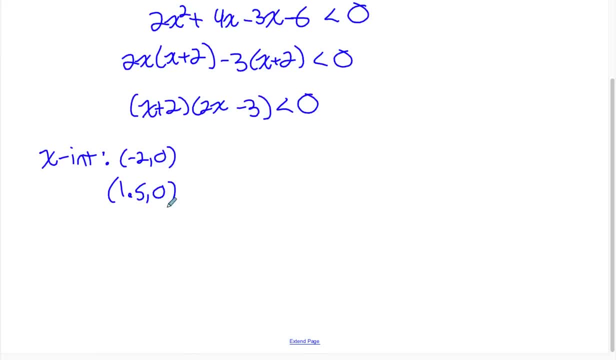 one point five zero. And this function, if we look back to the beginning of it, it had a positive leading coefficient, positive leading coefficient and it was even degree. So we know the end behavior of this function is going to be going from Q2 to Q1.. So if I made 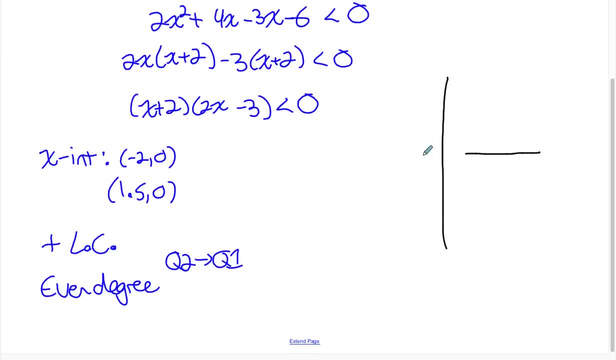 a rough sketch of this graph. I know it's going to cross, So this is just a rough sketch. I know it's going to cross the x axis at negative two and one point five and it's going to go from Q2 to Q1.. So it's going to look something. 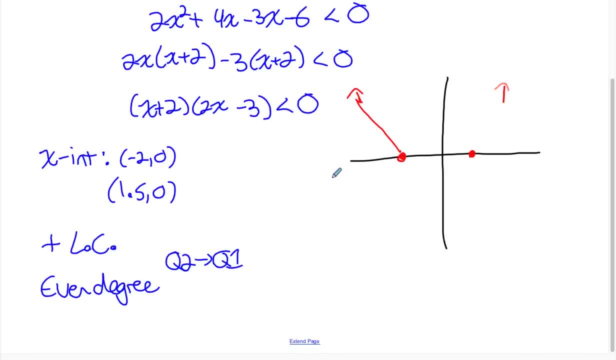 it's going to look something. Let me do a little bit better sketch of this. It's going to look something like this. So here's negative two. here's one point five, and we want to know: when is this function? less than zero? Well, it's less than zero. 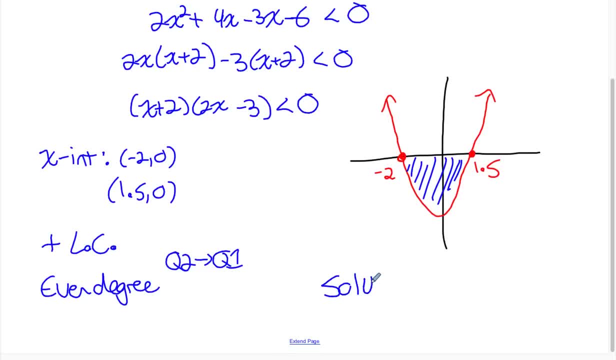 between negative two and one point five. So my answer, my solution, I'll write it in interval notation: My original function is less than zero when x is between negative two and one point five. So I write it like this: x is greater than two, but less than one point five. So that would be my solution. 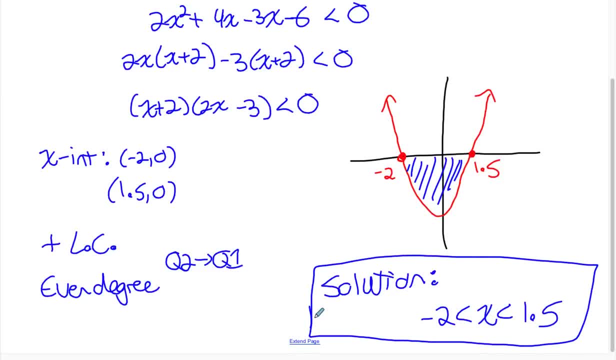 to this inequality. So just get it into factored form, make a rough sketch of it based on its end behavior, and then we can answer the inequality. 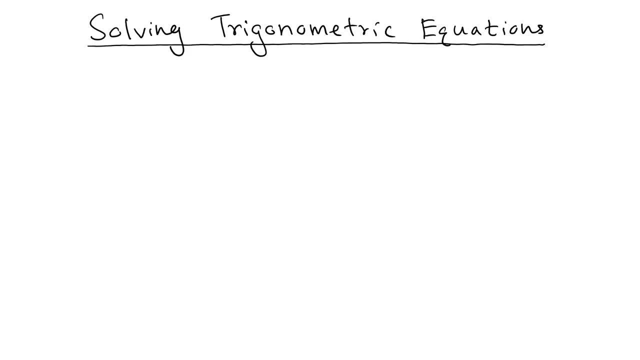 In this video, we are going to learn about one of the very important topic in mathematics. So we're going to talk about solving trigonometric equations. 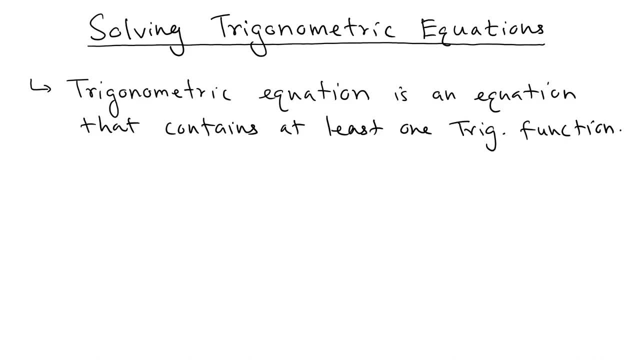 So what is a trigonometric equation? Trigonometric equation is an equation that contains at least one trigonometric function. So which is an equation which has at least one trigonometric 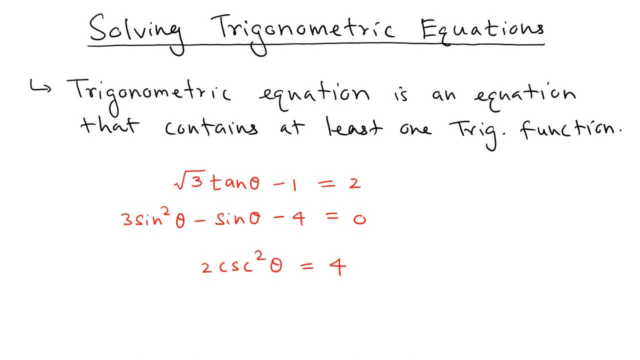 function. For example, these three are trigonometric equations. So you can say square root 3 tan theta minus 1 equal to 3 sine square theta minus sine theta minus 4 equal 0 or 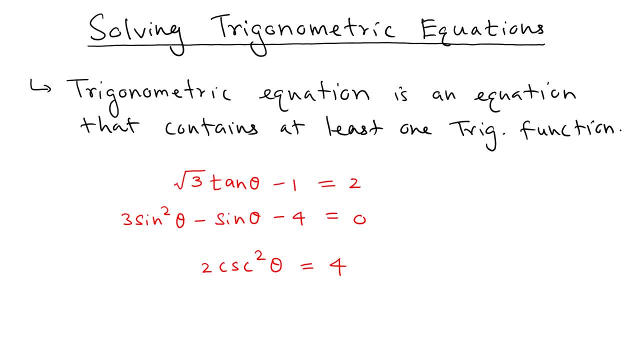